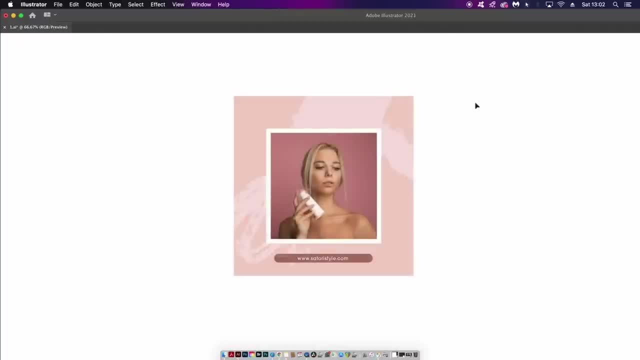 show you the finished design right now, and that is pastel kind of skin tones. as you can see, we have some darker skin tones here and then we go into pinks and also a really pale color here. so why are these synonymous with beauty products or skin care products? there are some very good. 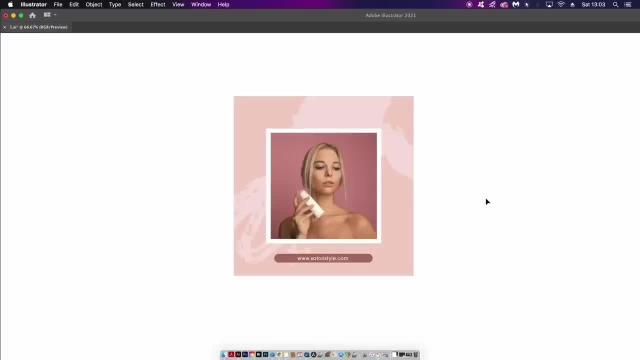 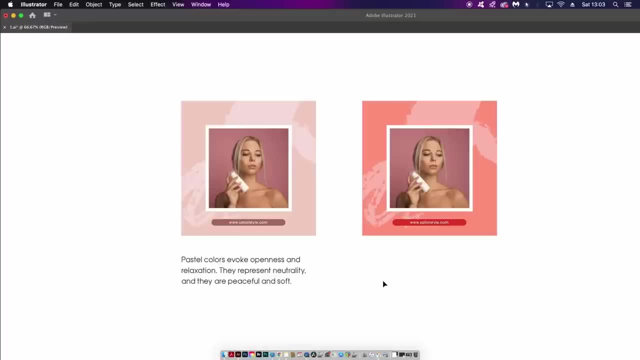 reasons why these kind of colors are used on these products. pastel colors evoke a kind of openness and a relaxation feeling when they're viewed. they're very peaceful in soft colors, which is great for selling things such as beauty products. as you can see on the right, the 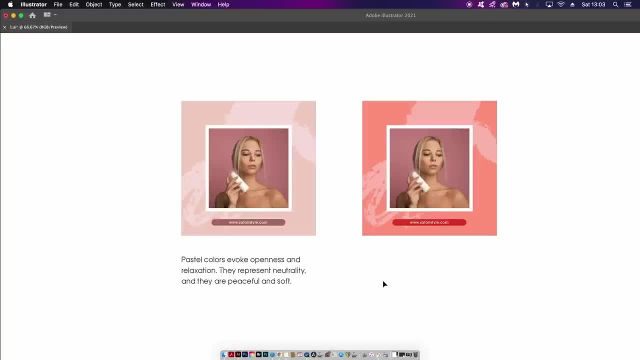 saturation has been upped a lot and it's too kind of aggressive for this style of design. also, using pastel skin tones does relate back to the product itself, which is trying to sell something that will make really healthy and really beautiful skin. so these are the kind of things you do need to keep in mind when you're 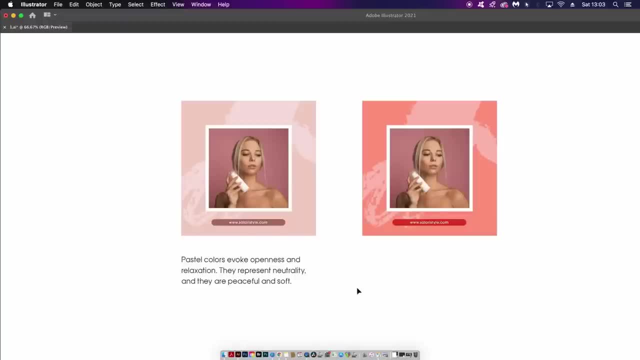 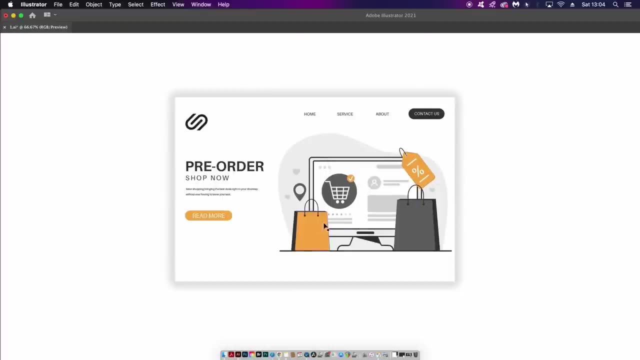 designing something you need to relate back to the product, the message and the overall feeling for this webpage. here i've gone ahead and i've actually colored in four aspects of the design in a kind of goldy orange color. the rest is grayscale at the moment, but we're soon. 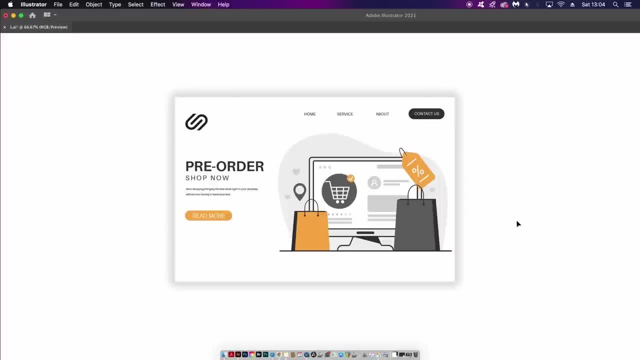 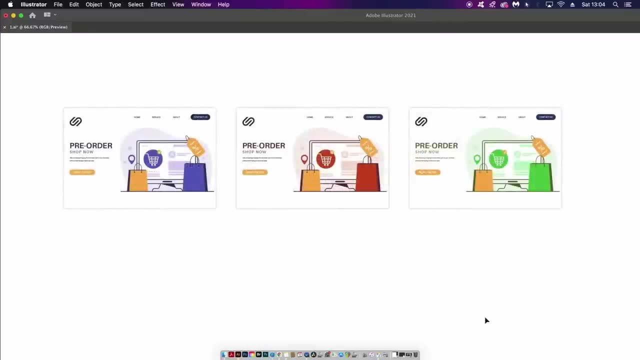 going to change that and actually i'm going to give you three different examples again and you should try and work out which one works the best for the design. so here are your three options to choose from. which design looks the most functional from a color scheme standpoint and can you actually answer why it works? this option is less to do. 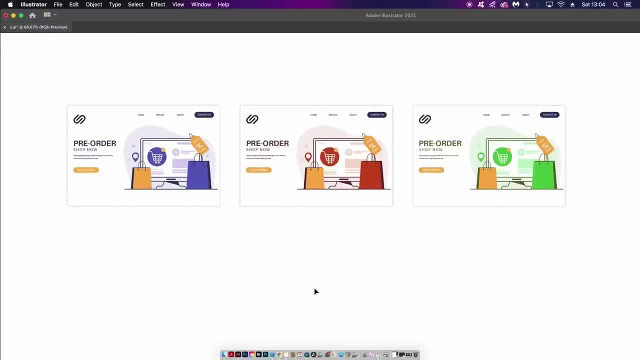 with emotion and it's more geared towards a graphic design principle in terms of color schemes. so one really useful method you can apply when choosing colors is to utilize contrast, and one really neat way to do that is complementary colors. now, these are colors that are opposite each other. 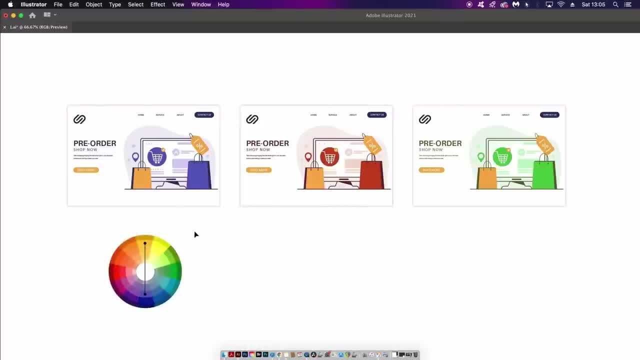 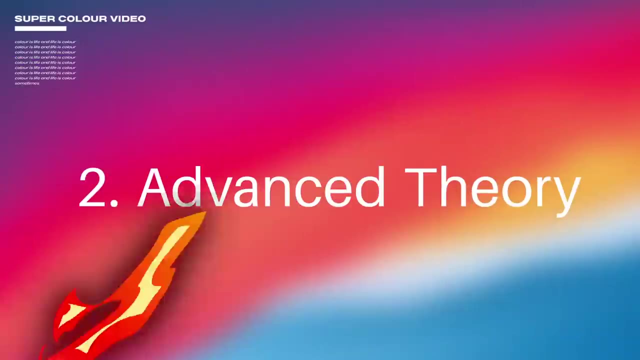 in the color wheel and of course, these are contrasting. this renders a design impacting, but also these colors are visually appealing when put together and this is something you might want to choose for your design when you pair it with things like emotion and the message. in 1974, kw jacobs demonstrated red to be more stimulating than green. 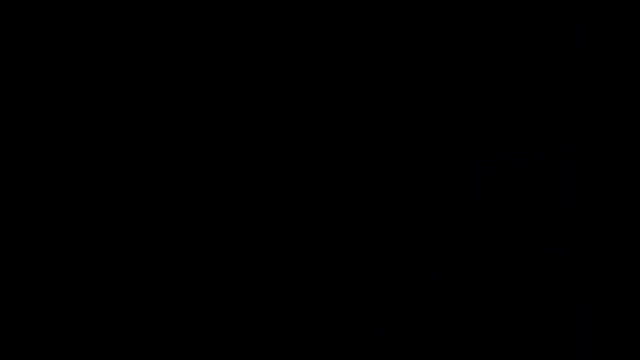 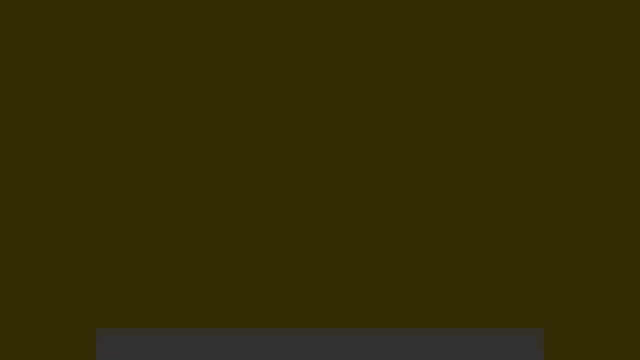 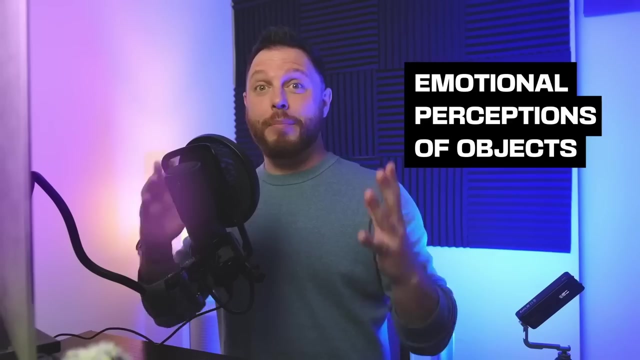 and green more stimulating than blue. according to this study, a person left in a red room constantly stimulated with heightened awareness and elevated heart rate, and in 1981 richard kuhler showed in studies that color had a great effect on eeg readings and heart rate, as well as emotional. 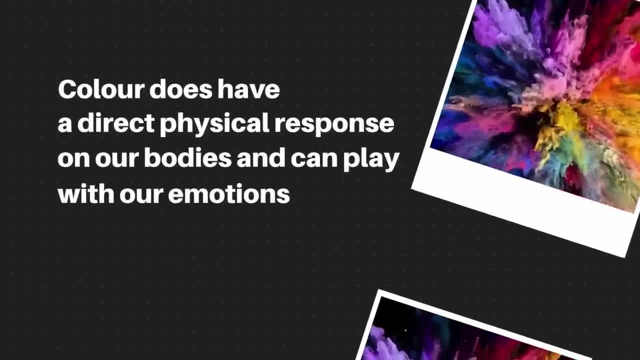 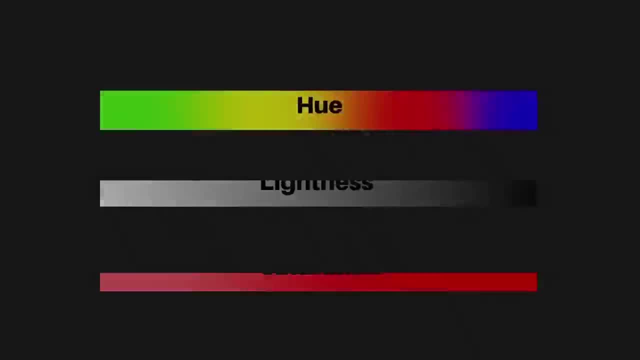 perceptions of objects. so color does have a direct physical response on our bodies and can actually play on our emotions. but here's the first very important thing you want to keep in mind as a designer: it isn't necessarily the color that's important. brightness and low saturation creates. a soft feeling, whereas dimness or lightness play a major role in any design. design is important and and a lot of things are still out there. even in the objects that we see here today, it's only important to carry color and all the models of color in close proximity, so color is not necessarily the best for. 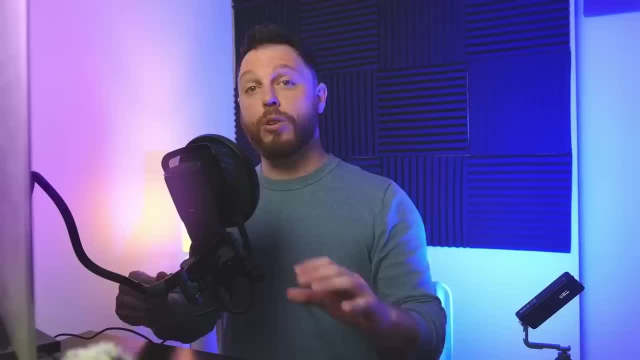 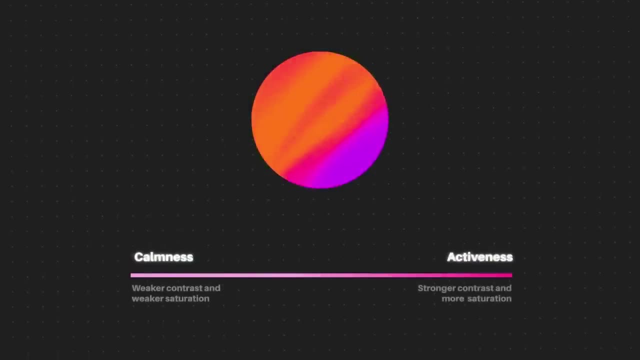 color design, but be aware that color isn't necessarily the best for each object in color and color is nothing to be, and high saturation creates a hard or strong feeling. Also, weaker contrast and weaker saturation conveys calmness, as opposed to a stronger contrast and saturation, which convey activity. It's why 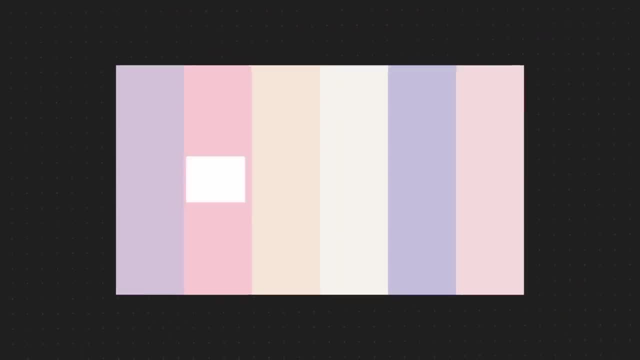 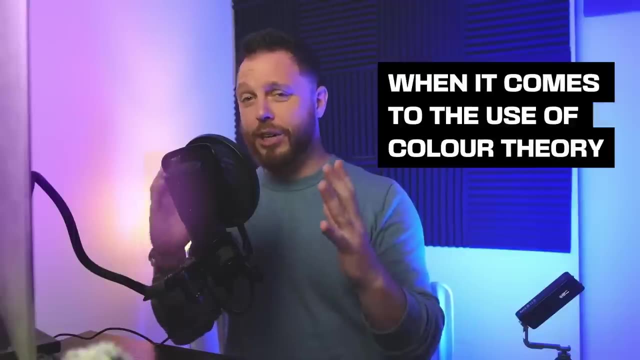 pastel colors are often given to baby things or are considered by some to be calming because they lack saturation And, as you can see, things do start to become a bit tricky when it comes to the use of color and color theory, but only if you don't properly absorb the content in today's video. 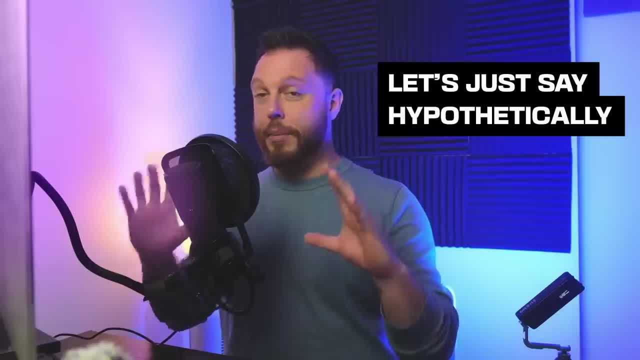 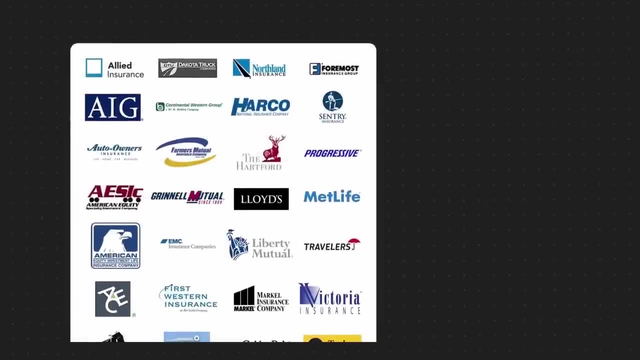 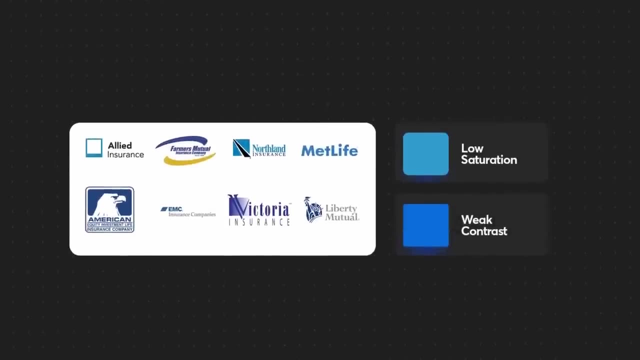 and potentially you do take some notes. Let's just say, hypothetically, we're making a design for an insurance company. Now, it could be a logo, a brochure, whatever it is. Using this knowledge, you might then choose one: low saturation, and two weak contrast. These decisions will convey a sense. 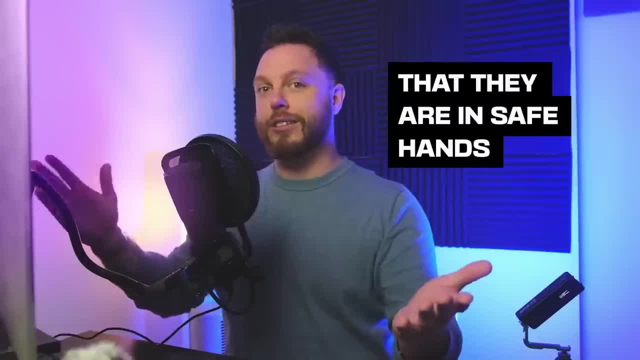 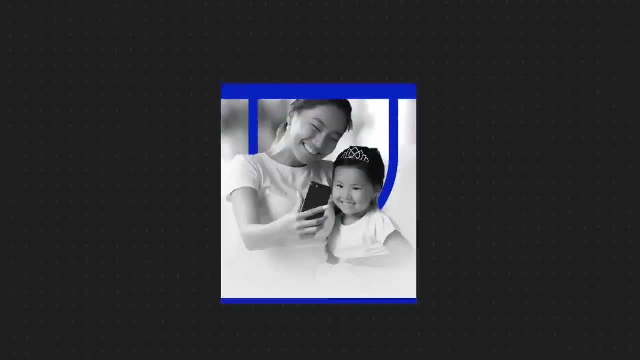 of calmness, which is great for conveying to the target audience that they're in safe hands and that, yes, they will purchase 100 years of your finest insurance. Knowing the message or feeling you want to send out with your content is a great way to convey calmness. 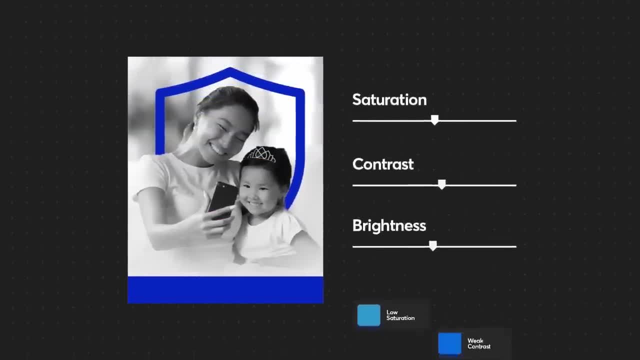 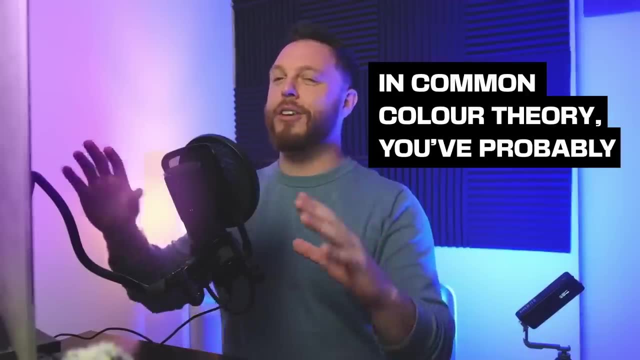 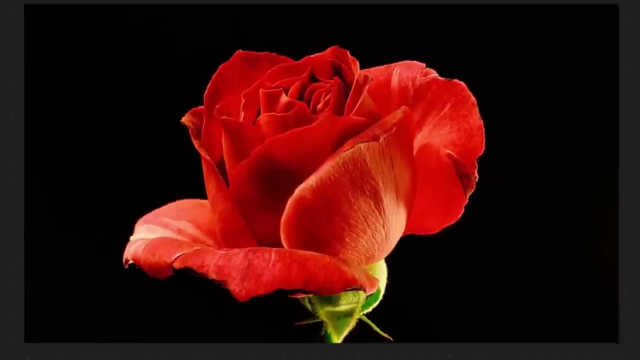 But let's go deeper with color theory. even yet still In common color theory- you've probably heard this a thousand different times- The color red relates to danger, but also to passion and lust, blah, blah, blah. Yes, to some extent this is true, of course, but get this. we already know that from 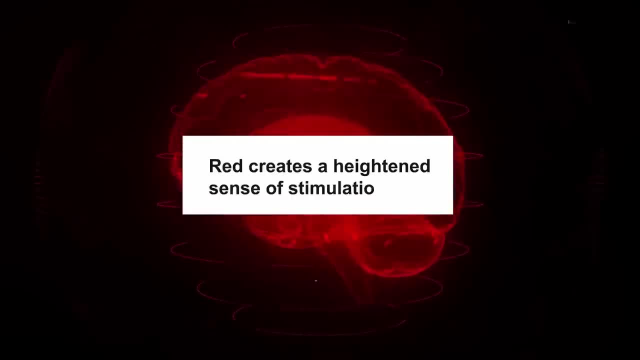 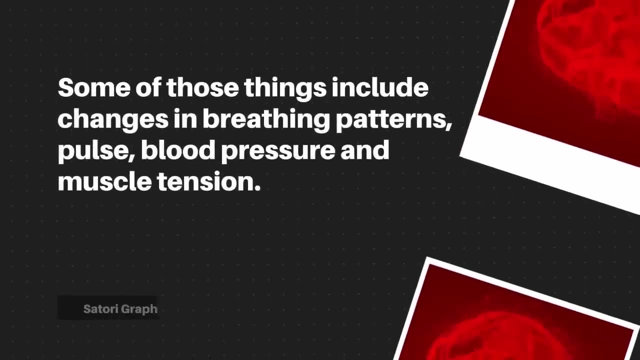 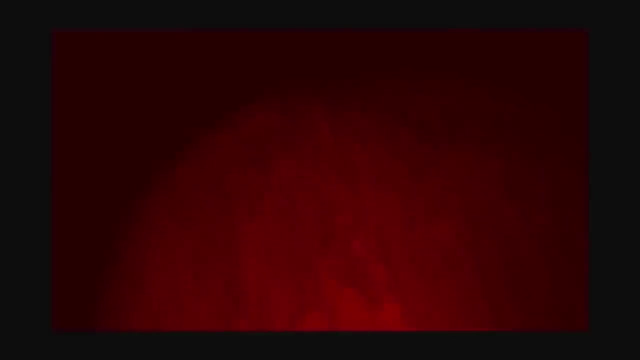 the study mentioned earlier that red creates a heightened sense of stimulation. Being stimulated like that does a few things. Some of those things include changes in breathing patterns, pulse, blood pressure and muscle tension. Okay, cool, but where does that even fit into graphic design? So when people are at this, 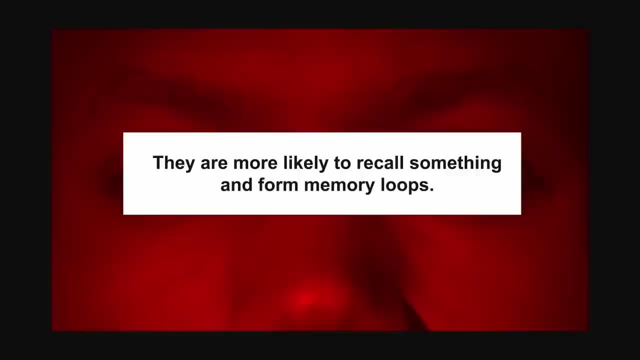 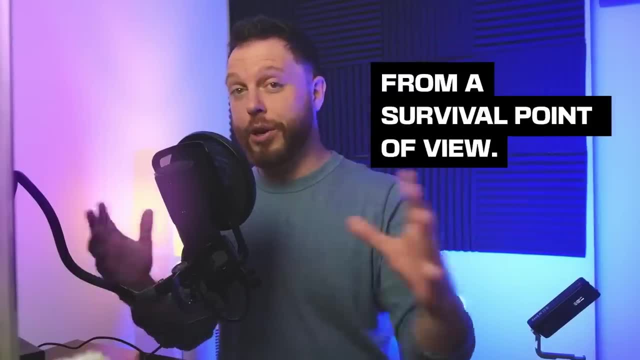 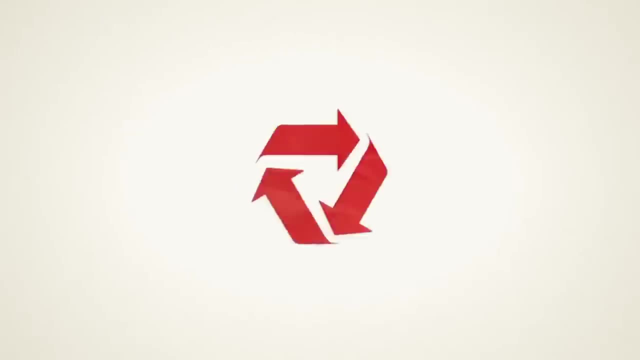 level of stimuli, they are more likely to recall something and to form memory loops. It's like mini trauma and our brains are designed to latch onto trauma. from a survival point of view, Many brands and many designs use red or similar colors to grab attention and to create hard. 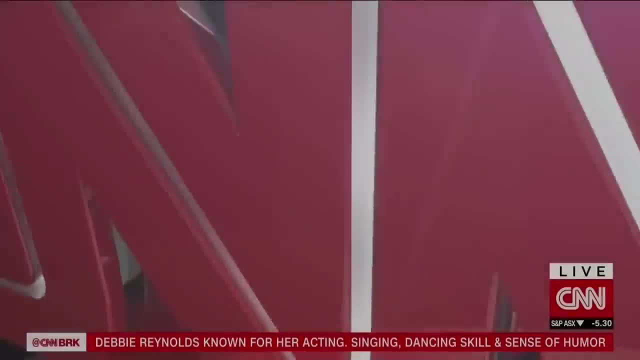 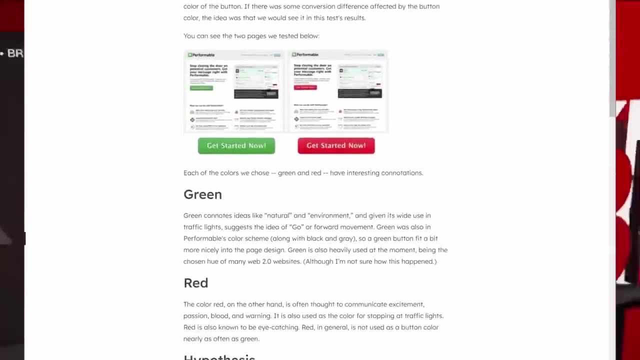 solid memory. So when people are at this level of stimuli, they are more likely to recall something and to form memories to their audience. Think of brands like CNN or Target as example. So for the UI and UX designers out there, Hubspot ran a study on the effect of switching website. 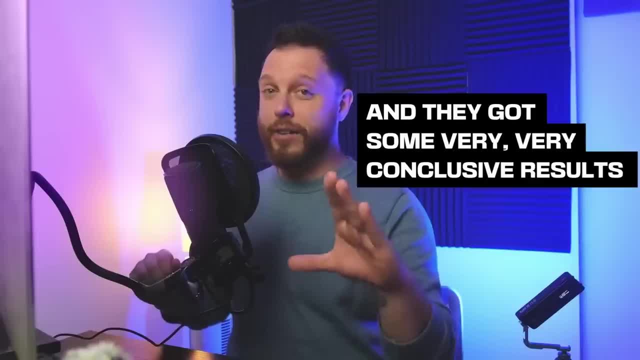 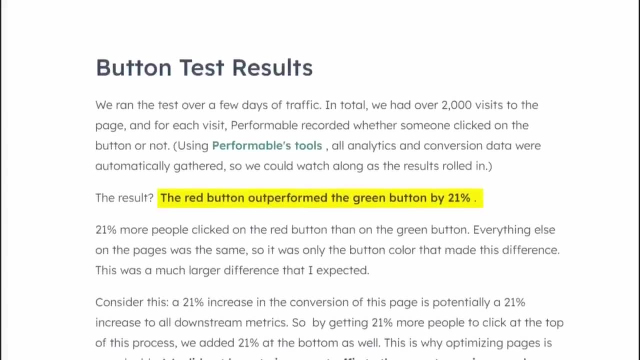 call to action buttons from green to red and they got some very, very conclusive results. The red button outperformed the green button by 21% in terms of click through rate, Which is pretty major in the business world. Color theory can be fiddly and it can be precise. 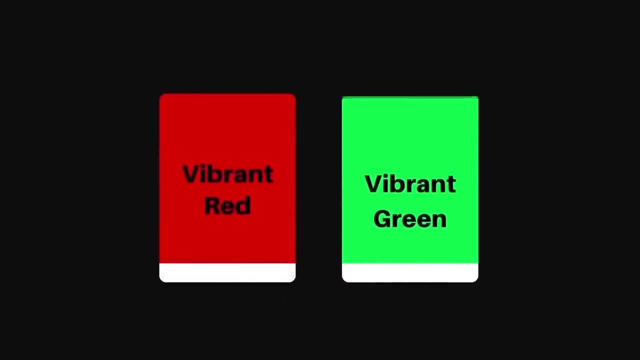 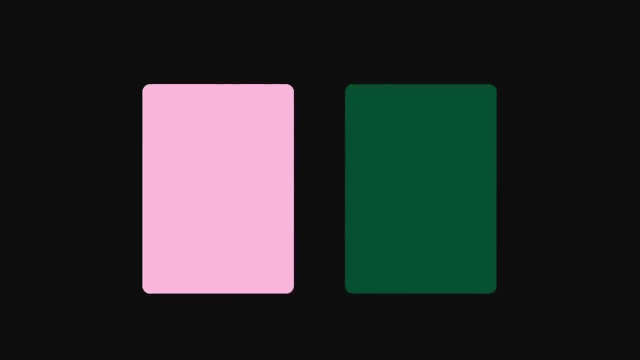 at times, For example, Lighting a vibrant red and green together can end up being unpleasant to the eye, But if you lighten the red to a soft pink and then make the green less saturated and slightly darker, it then becomes a decent color palette, One that is immediately memorable and visually 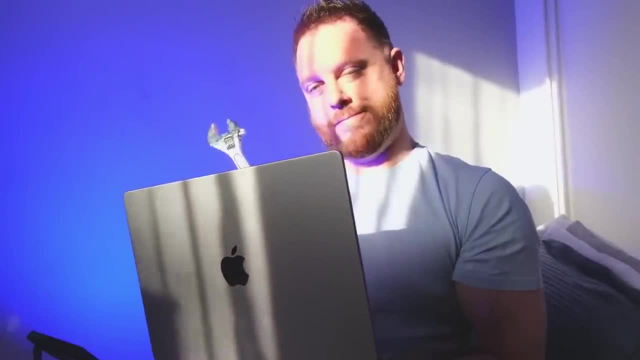 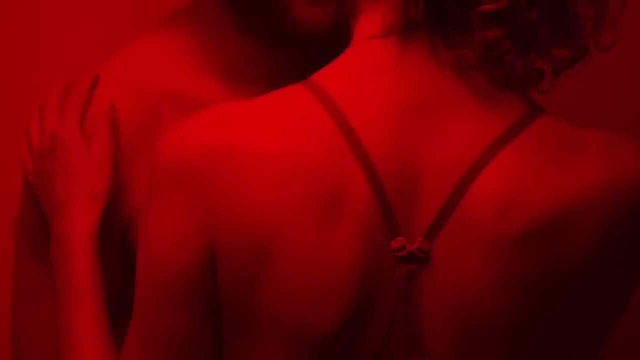 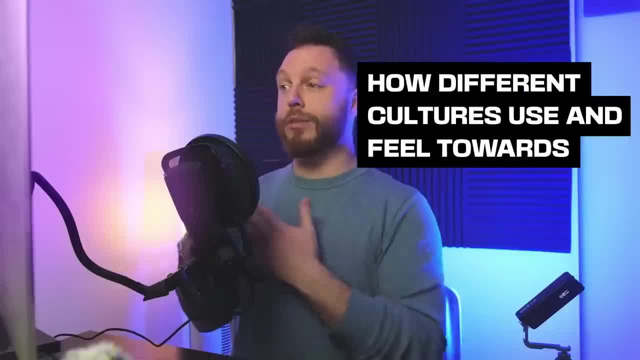 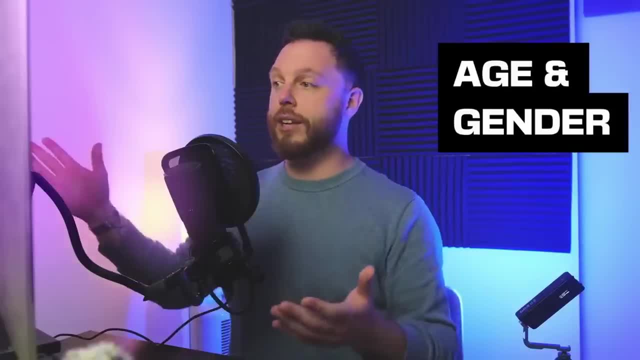 associated with red. There are many different examples of how different cultures use and feel towards color, But here's yet another spanner to throw into the works. Age and gender Studies have shown that women tend to prefer softer, more pastel colors, Whereas men prefer 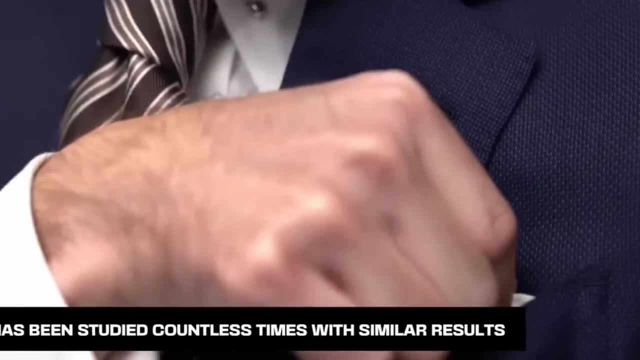 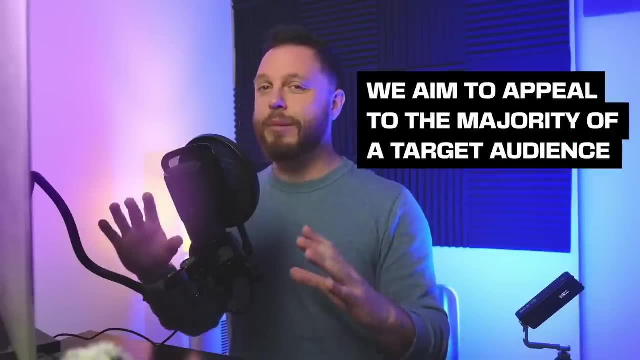 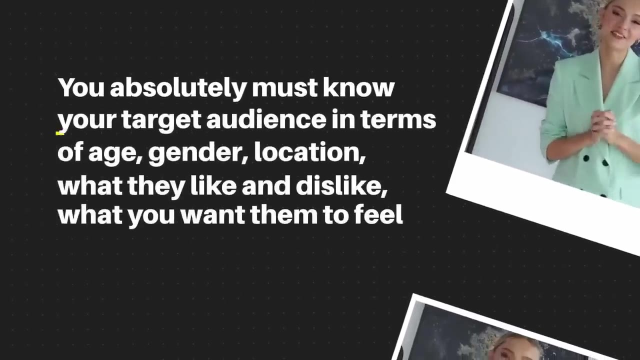 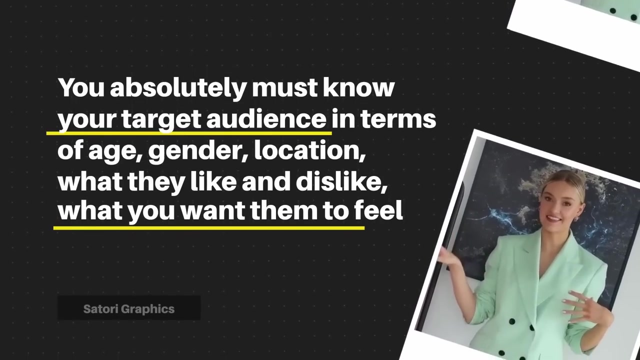 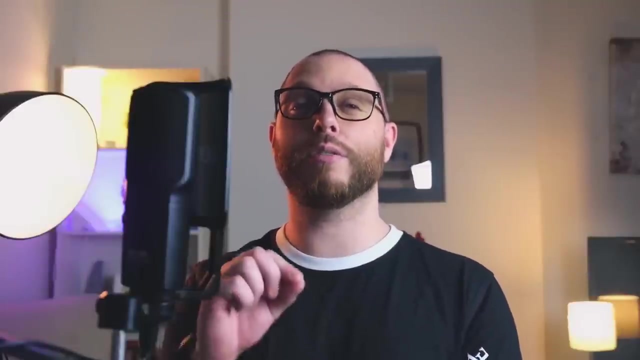 bolder colors. It's important to note that this is just an average and won't apply to everyone in a group, But when making designs and decisions on those designs, we aim to kind of appeal to the majority of the target audience And for this first section, you're going to want to write down words linked back to how. 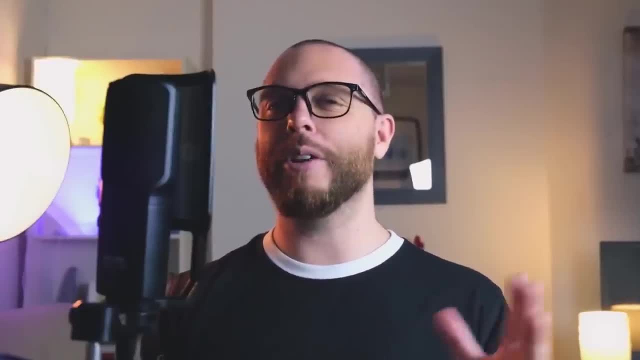 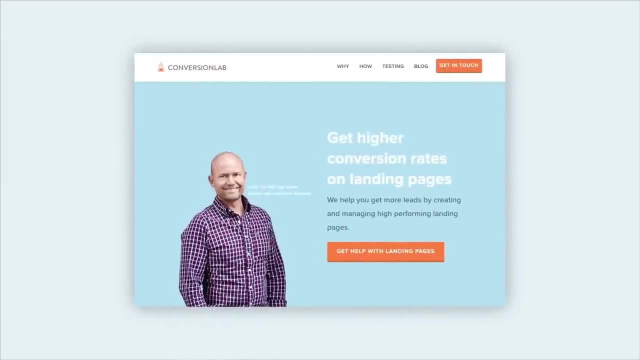 you want to make the viewer of your designs feel- And don't worry if you're kind of lost, it is going to make sense later in today's video Existing examples. So this landing page wants to make the viewer feel like they are in good hands. Notice how. 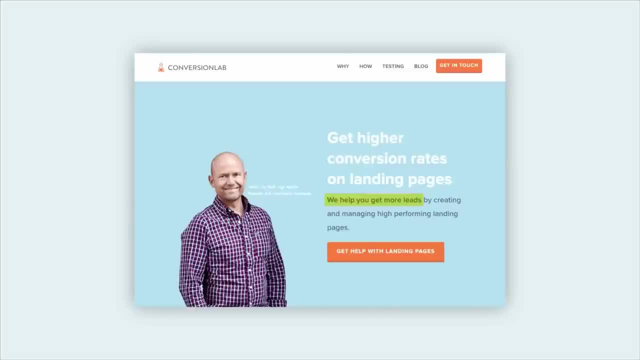 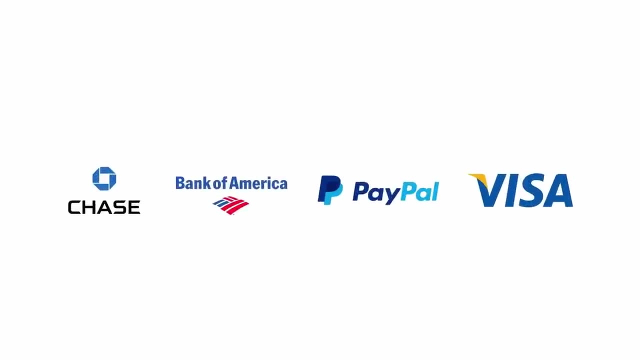 it says: we help you get more leads. Emphasis on that word help. Blue colors are strongly linked to a sense of security and it's why most financial based brands use blue in their branding, But a light and a soft blue like this one here is also. 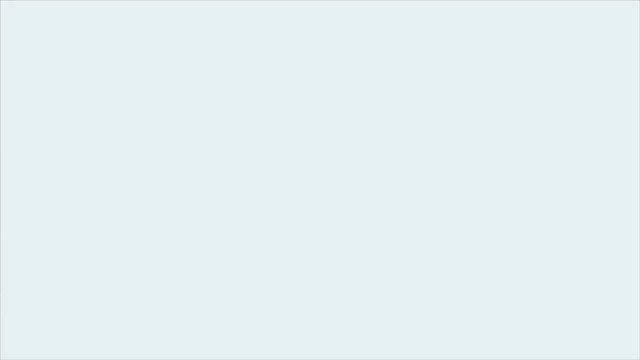 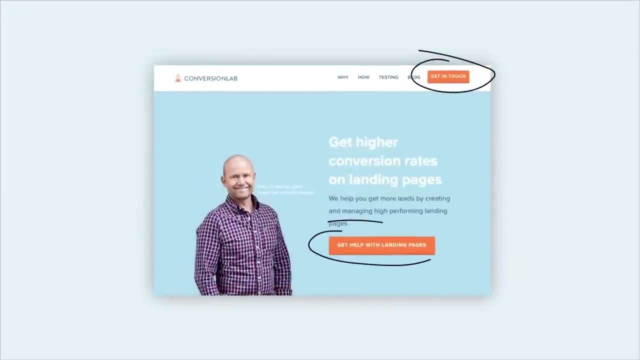 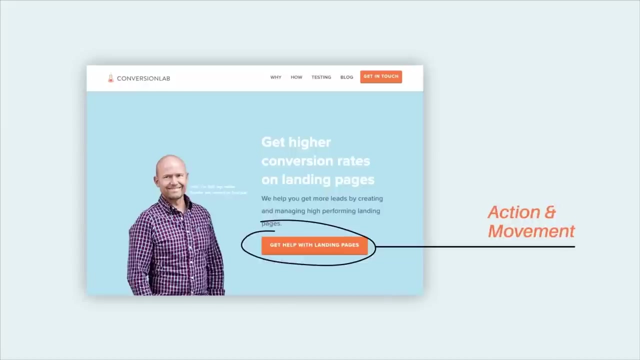 quite calming, So the words you might write down relating to how you want the viewer to feel are safe, secure and calm. Notice, however, that we also have hints of orange on our design. Orange is a color linked to action and movement, and so this will help to usher the viewer to take action and click. 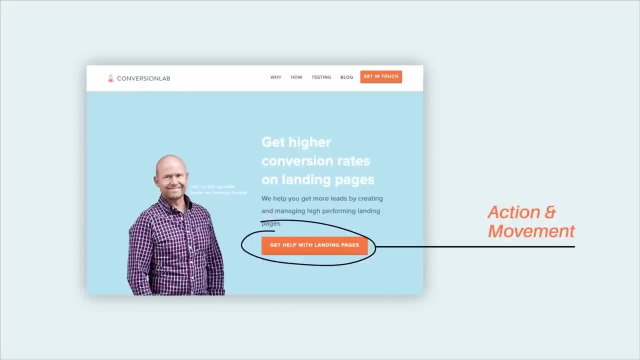 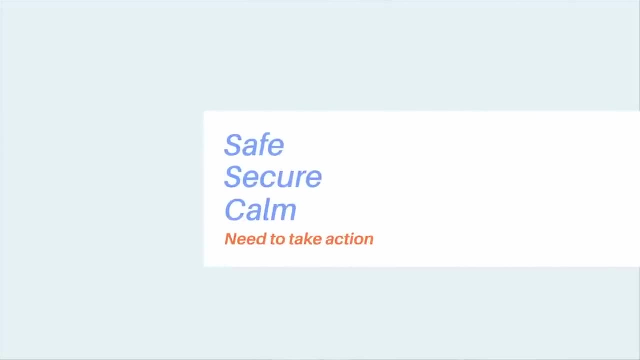 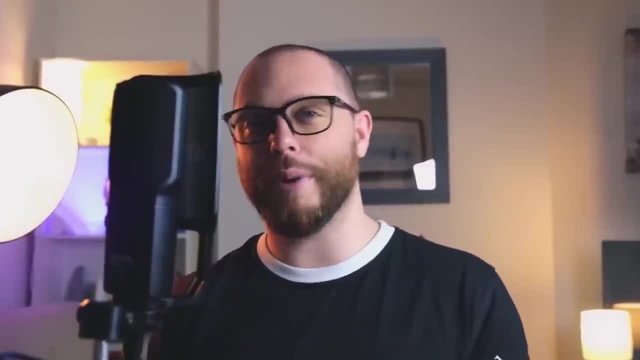 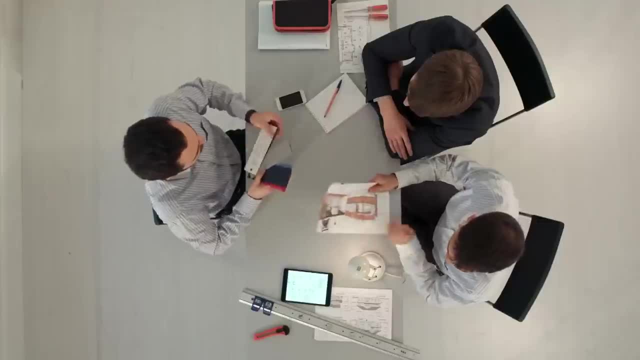 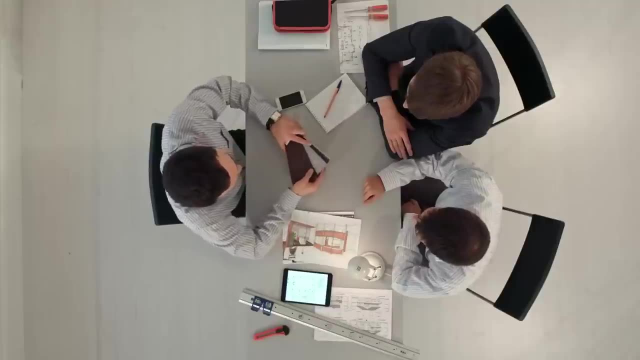 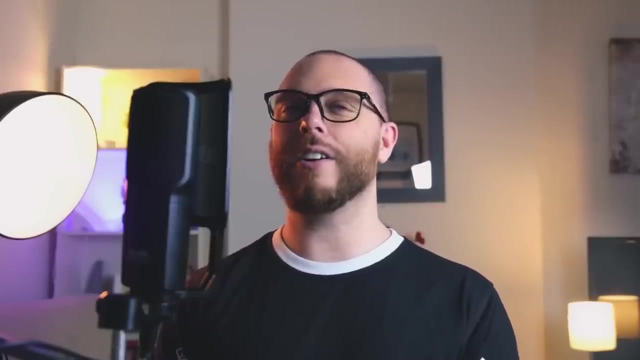 useless. This is a clearly ignorant standpoint because psychology, especially in terms of color, is used by pretty much every major brand out there, Not to mention that color psychology is something ingrained into the human brain and also into cultures around the world. So to say that color psychology is rubbish or useless is very, very ignorant, and it's just. 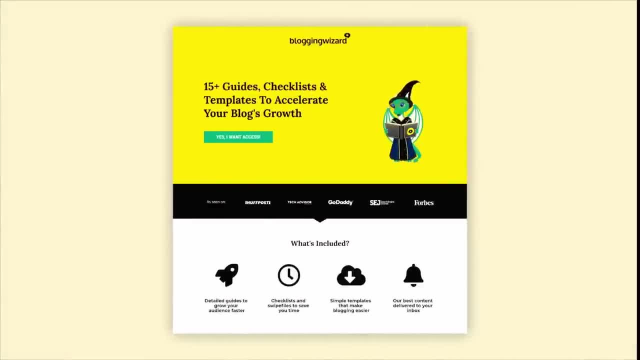 redundant, to be honest. Let's look at another quick example for this section. Let's look at another quick example for this section. This design wants people again to feel energetic and to take action. It says: accelerate your blog's growth. That sentence not only suggests the viewer to actually do something right. 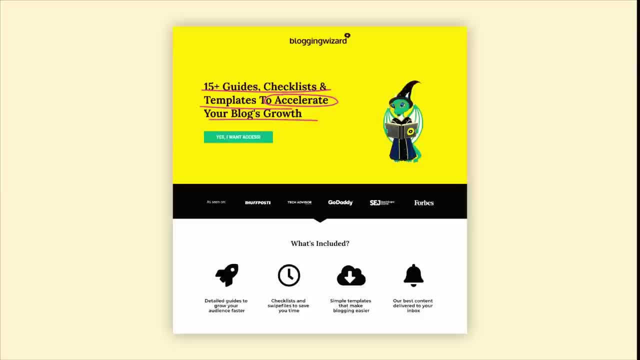 now the word accelerate is in there, which in and of itself is very energetic, And again a strong, bright color of yellow is used in this design, and this time it's the main color, unlike the touches of orange we saw earlier. Yellow is linked to energy and positive change. 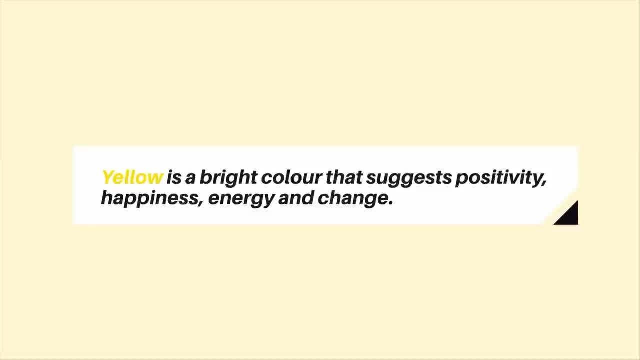 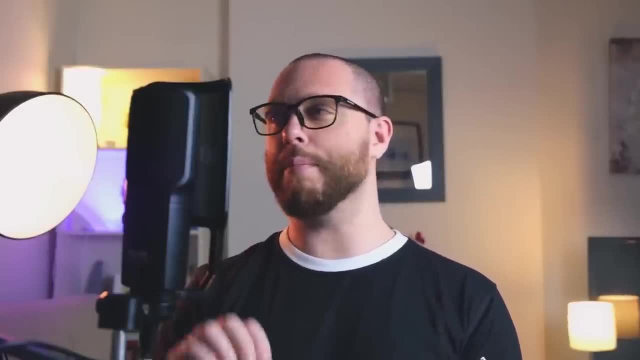 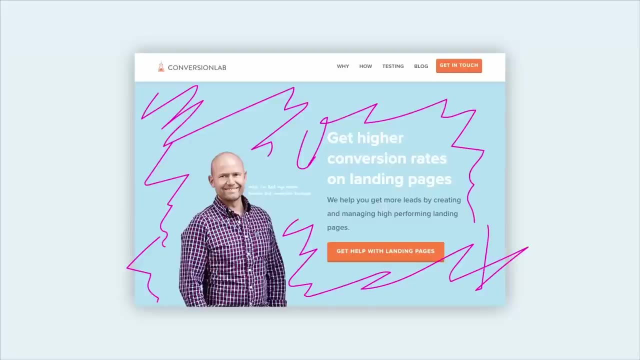 much like orange, And this is no coincidence. It's color theory and psychology. The next step is to look at your designs- personality- and again we want to write down those words that best describe the personality of your design. Let's look at this design again and there is a lot of white open space, suggesting a 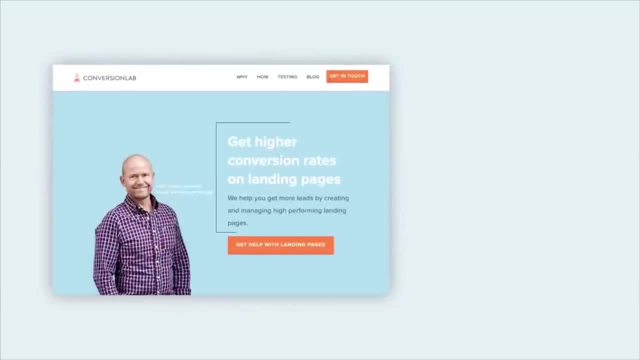 more minimal and a more clean design. The fonts used and the style of use is quite friendly, especially considering we have a little message in handwritten text next to our model For this design. I would write down a clean, minimal and friendly and add these below the first section of words that we've made. 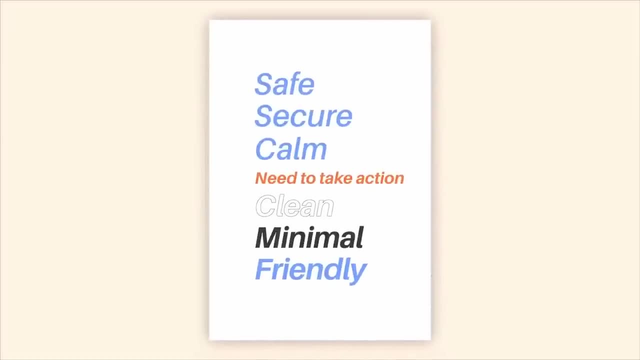 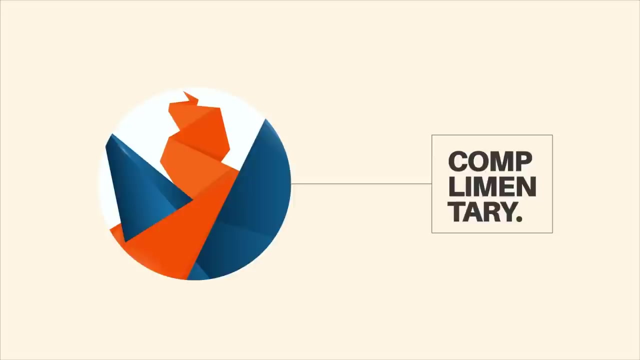 We want to build an overall idea or concept of our design with these keywords From here. it's a case of just taking your words and thinking about color psychology. So pop online and take a look at what each color signifies from a psychological point of view, and then match up your keywords to one, two or three colors. 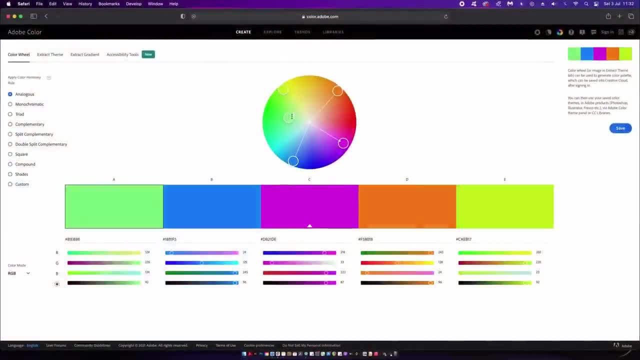 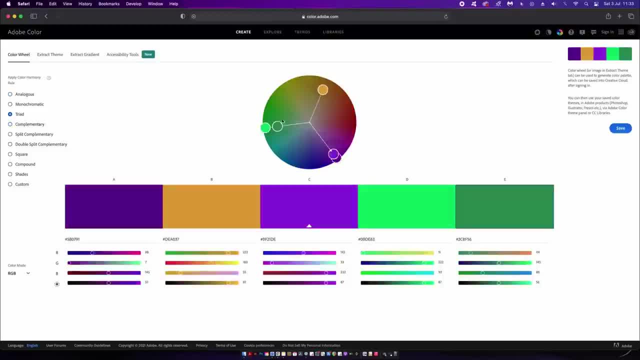 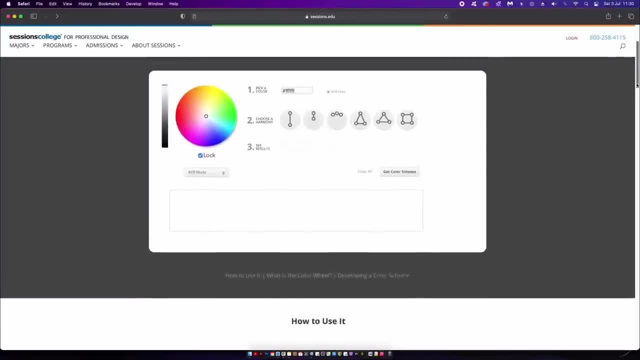 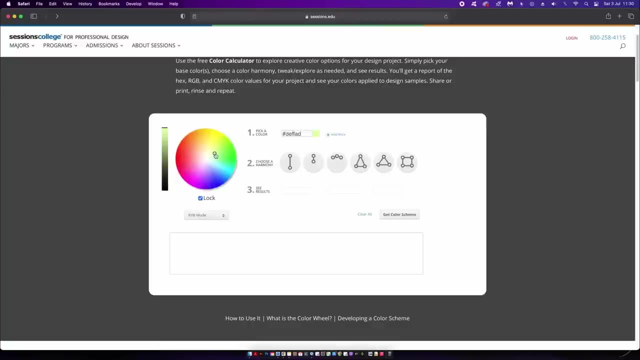 Which is a color scheme? I'm sure you've probably heard of Adobe Color. Let's just say, for example, that your research has pointed you in a direction of a friendly and natural organic design, So you want to go for a muted kind of tamed green. 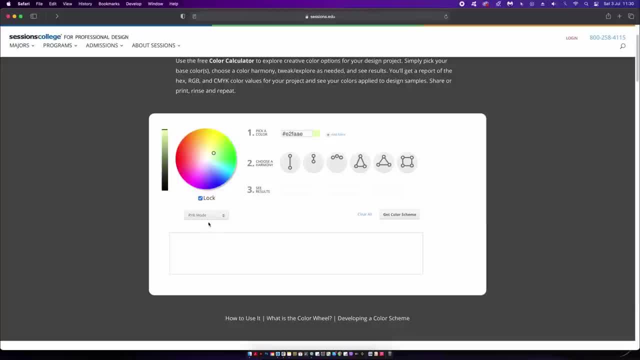 This is your starting color. This is your base color. You can then cycle through different color harmony schemes, such as complementary, monochromatic and so on, with that base color from your research and then explore what else can work and then what might fit into your design. for example, here the green could be the majority of my design. ie that main. 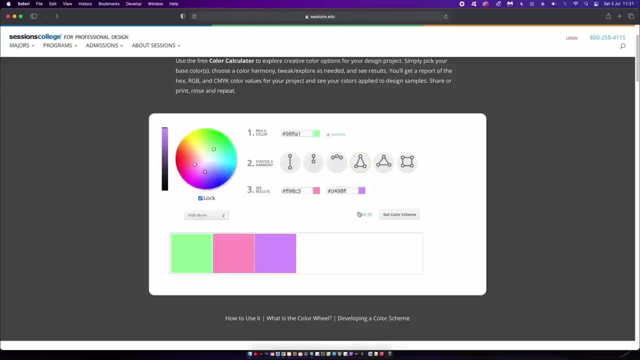 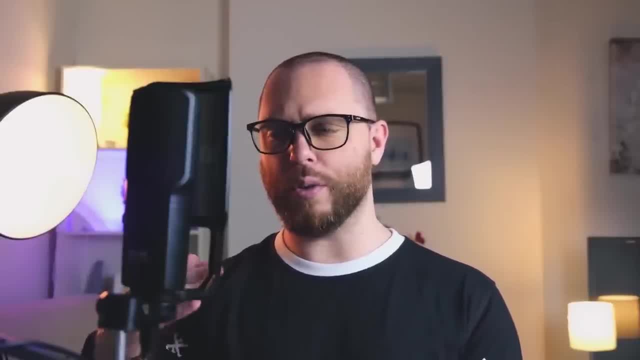 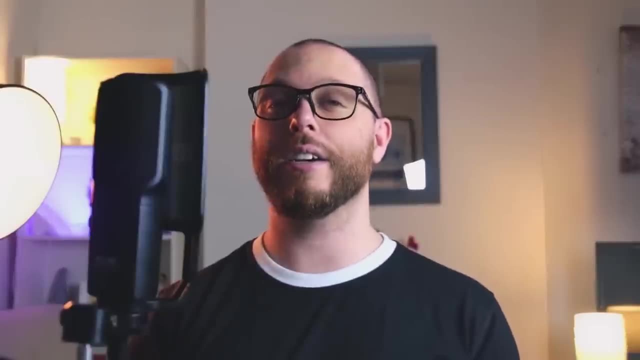 color, and then maybe this pink or this orange could be the call to action, focal points and other design elements. so this is how we do it: we first want to think about the viewer and how we want them to feel with our design, and then we think about the design's personality before methodically. 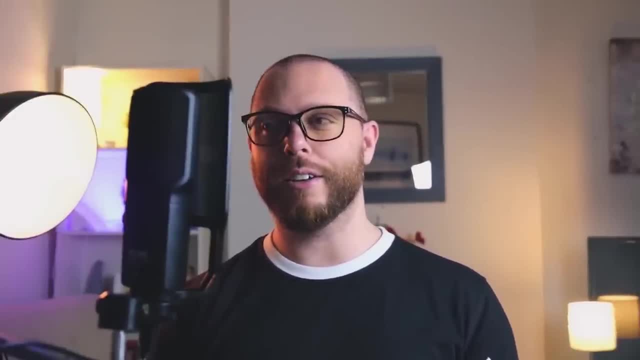 going about the color scheme itself. sometimes, when you're lucky, the brand or the client will give you a color scheme and then that means most of the work is already done for you. but i hope you see how design can be a methodical, step-by-step process. and yes, it's creative, but it also requires 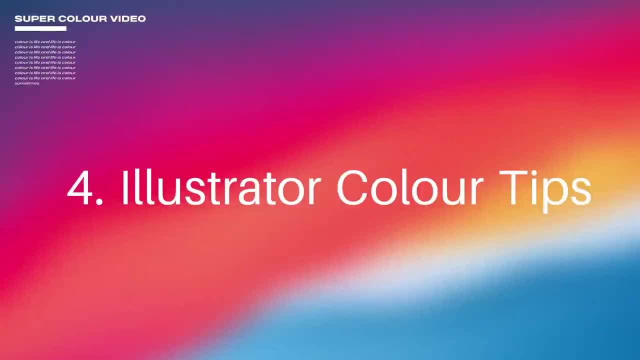 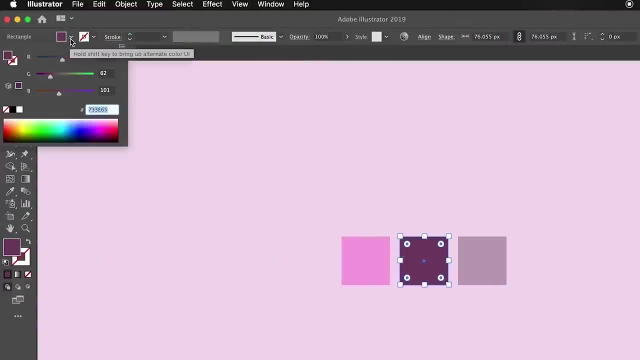 some you know methodical thought as well. one thing you might not know about illustrator is that if you hold down, shift and click the color menu, a different menu is actually presented to us. now i'm currently working in rgb, so i do have the relevant rgb sliders, but if i then hold down, 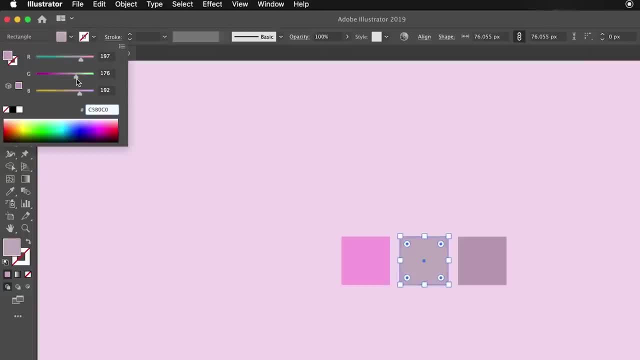 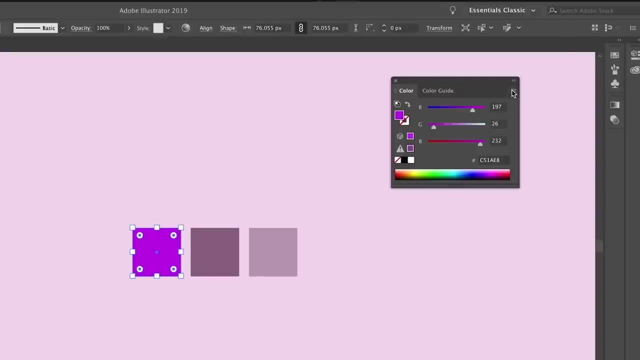 the shift key again and click and drag. notice that i'm actually dragging all three sliders at the same time. this is actually a quick hack to add tints and highlights to your color straight from the rgb slider panel, which is pretty neat. also when we take the color window, something 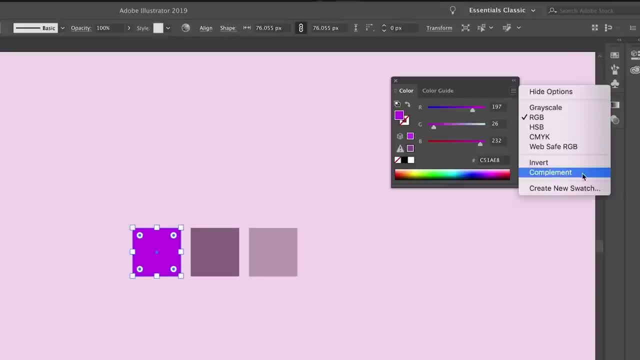 that is often overlooked by some people is the ability to complement a color straight from this panel. this, of course, refers to the complementary color scheme, where opposite colors on the color wheel are paired up together. so, for example, if i take this blue here and i use a complement button, we should get an orange. another nifty and time-saving tip in illustrator: 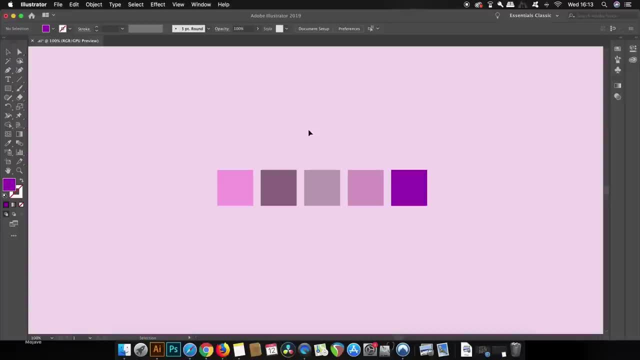 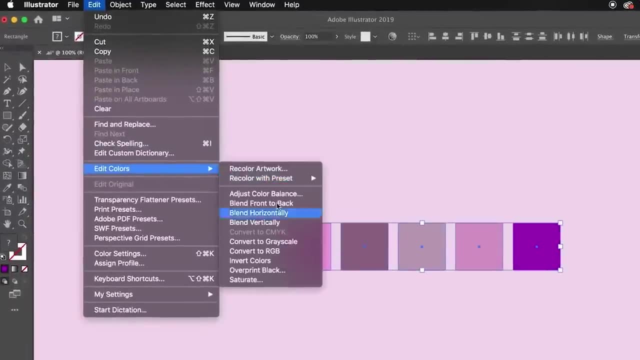 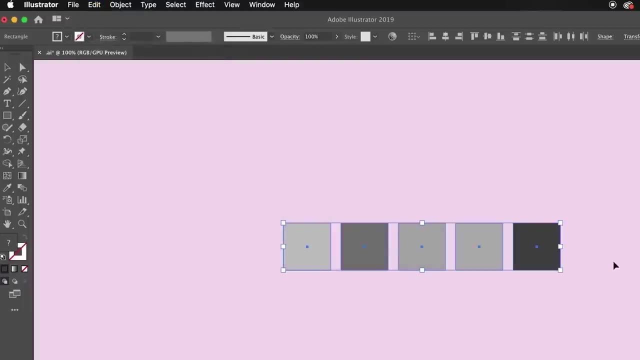 is a way to change an entire design color scheme with just one click. make sure you select everything you want to change and then come to the edit colors menu. here we have a lot of color options, such as grayscale, saturation and so on, and, as you can see, i now have a totally grayscale selection with just a single click, one of the most. 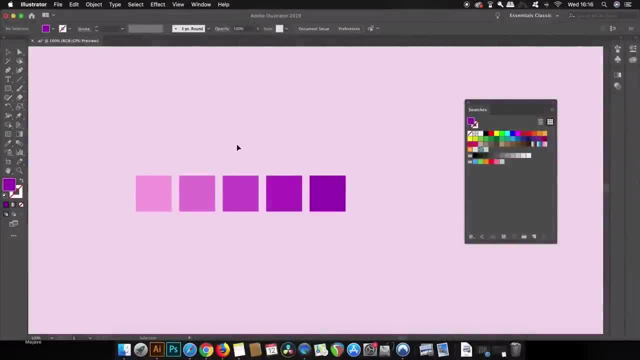 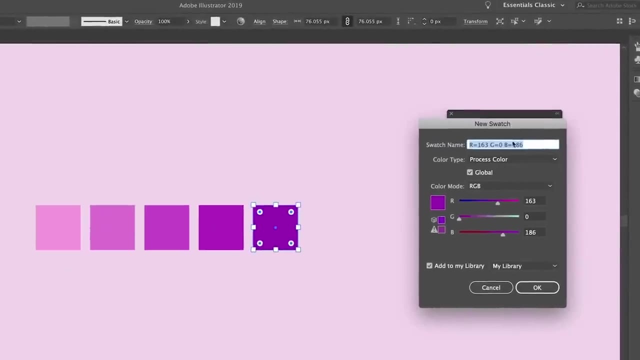 powerful ways to use color in illustrator is to focus on global colors. to use this option, open up the swatches window and then select the base color that you wish to use as a global color. then click the top right menu and add a new swatch. make sure the global color box is checked and once you've made the swatch, 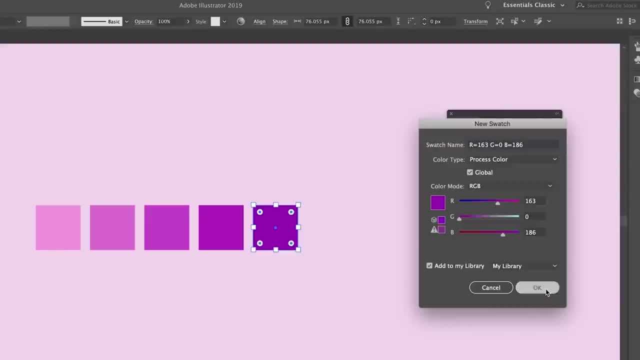 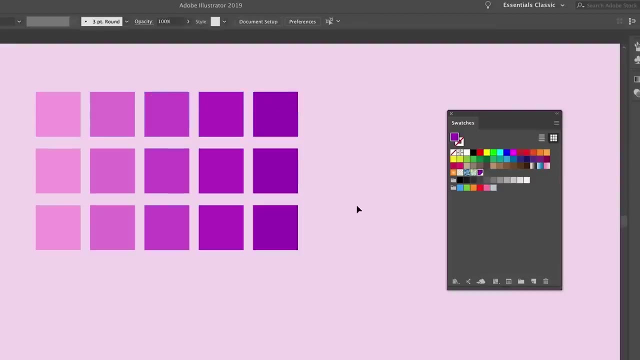 you will notice that the icon has a white triangle in the corner. this is now a global color. this means that whenever you use this specific color on your project and then you come into the menu and you edit it or transform it into a different color, it will actually change across your entire design simultaneously. 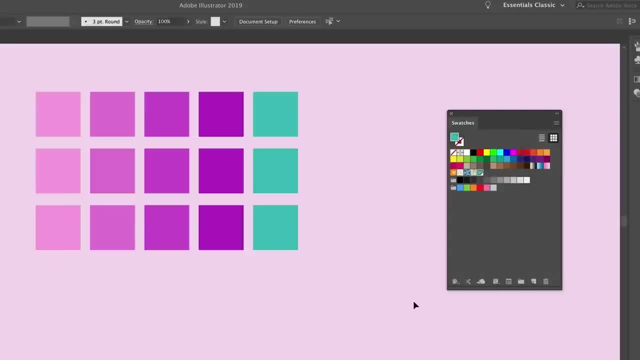 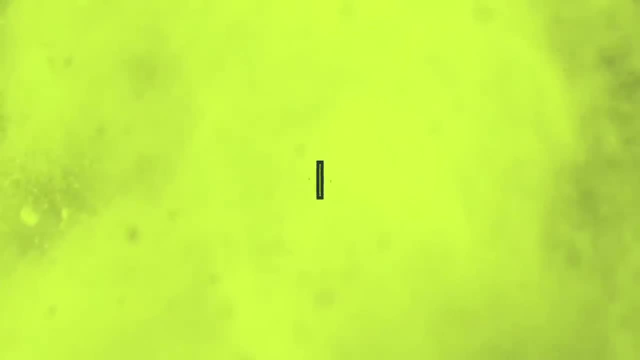 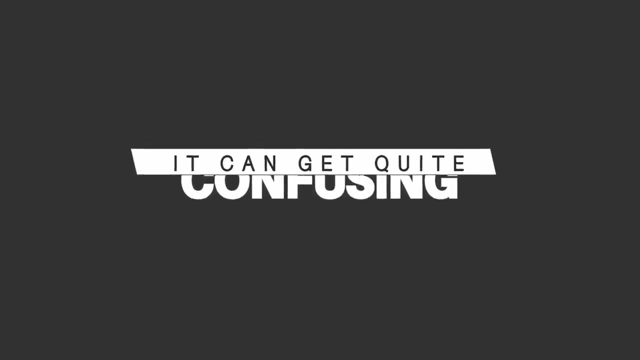 now you can even change the optimal color from color biology to any other color in the design. now pretty much everybody has heard of color psychology and the rules attached to that psychology. but do these color rules really mean anything in business and branding? well, yes, they do, but it can get quite confusing. 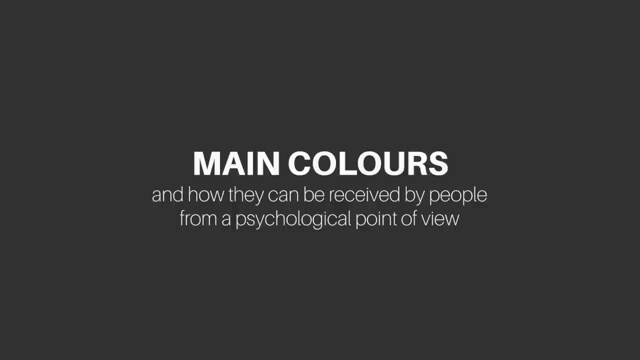 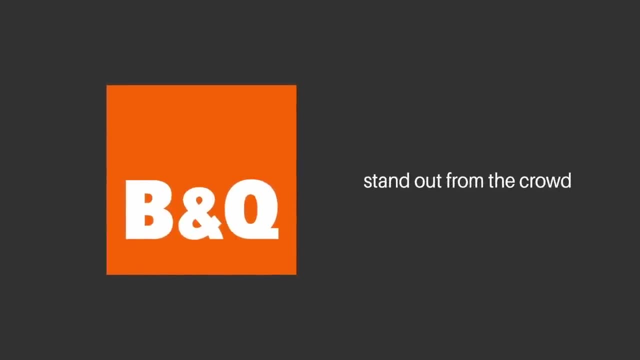 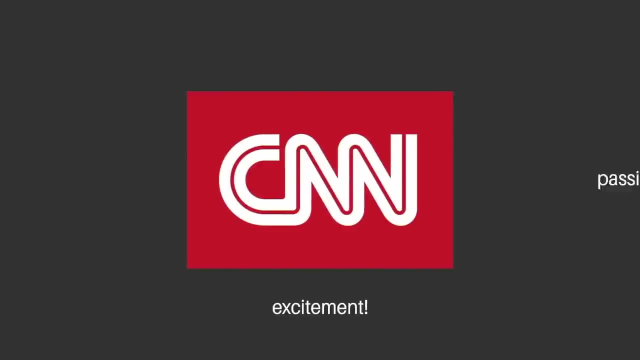 let's start with a simple by people. from a psychological point of view, orange is an invigorating, playful color, and it's one that will make your logo stand out from the crowd, and it's often used to represent a positive change or action and energy. red is the universal sign for excitement, passion, but also anger. now. 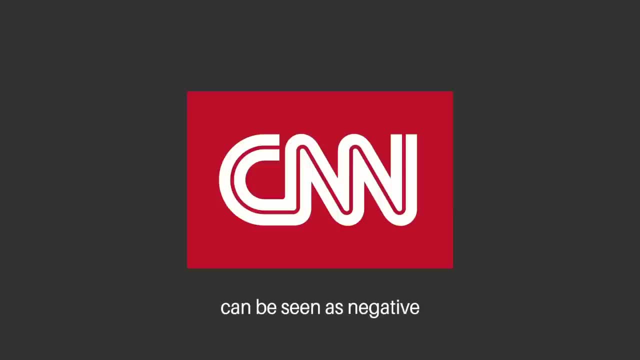 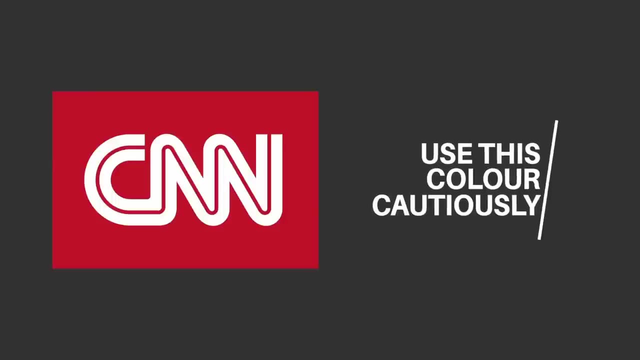 like orange. it will stand out from the crowd, but it can be seen as a negative kind of connotation in some cases. it's a color to be used cautiously and, don't worry, we're going to look at things in greater detail later in the video. this is just a quick rundown of the colors, if you want to. 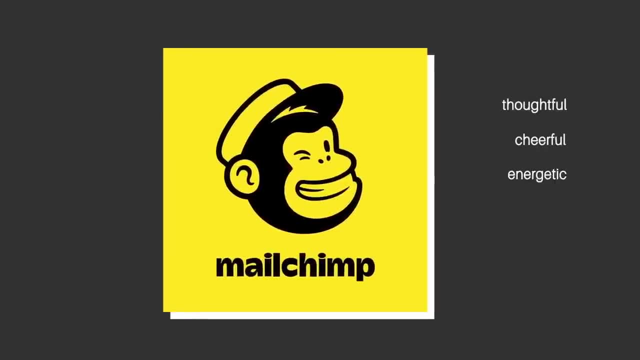 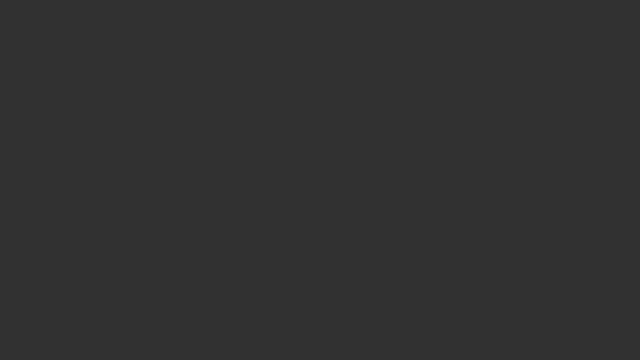 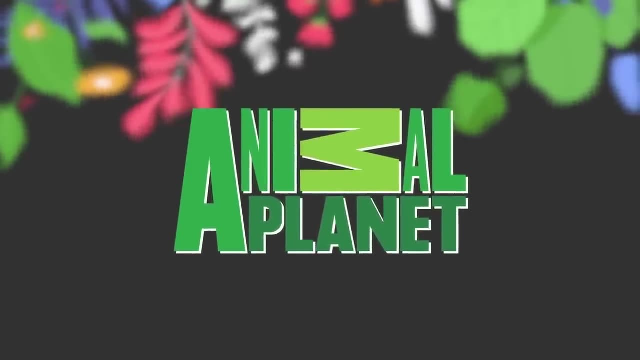 interject a thoughtful, cheerful and energetic emotion into your brand or your logo. yellow might be the way to go, and again, this color is very loud. green is very straightforward because it represents nature, growth, health and it can be used in almost any sector of business. you blue symbolizes trustworthiness and maturity. now you should be using blue if your brand. 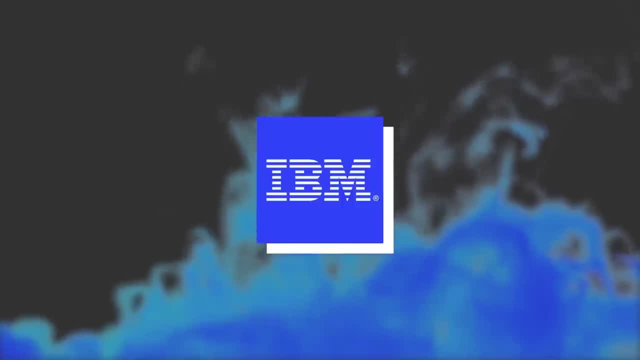 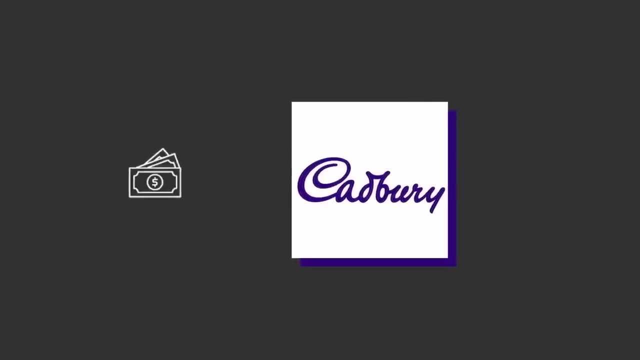 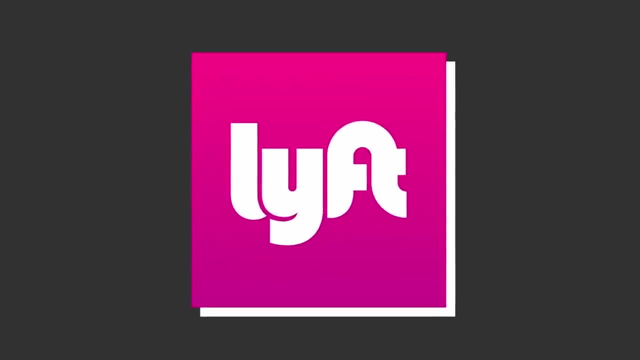 wants to be taken seriously. it's also a color that can be quite calming. now, purple is feminine, but it also expresses luxury and it's often the color linked back to royalty. so, in short, it's a pretty sophisticated and feminine color. in western society, nothing says girly like pink does, but it is a lot more versatile than that. and now, if pink is a more? 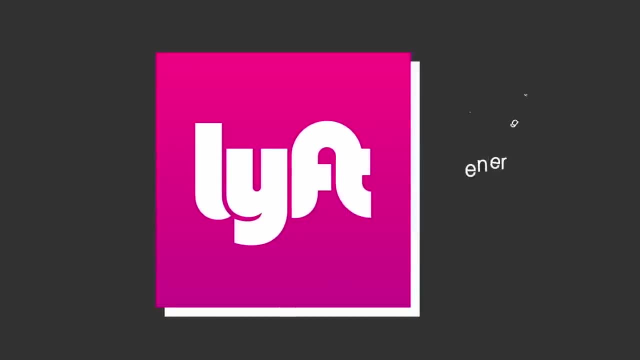 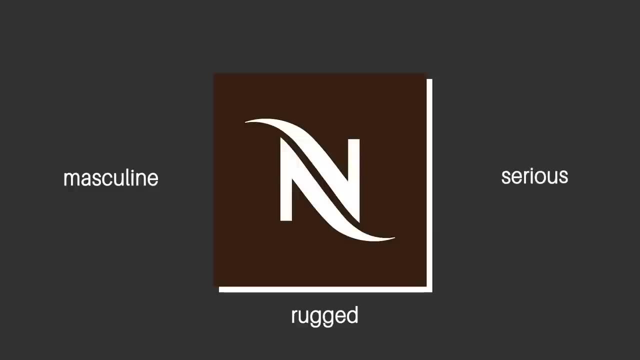 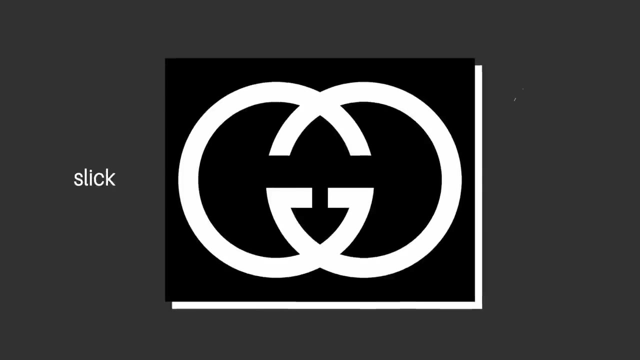 vibrant neon version of its color, then this can represent energy and a more modern emotion. browns will often make your logo appear rugged, masculine and also serious in nature, but browns are rarely seen in logo design. black can be slick and it's a modern and luxurious color to use on. 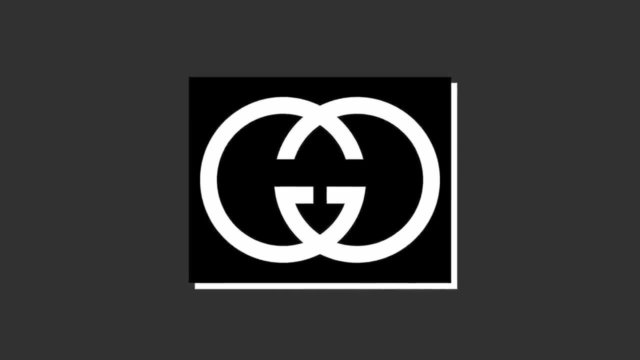 the logo, and it's often used for high-end brands. ie nine just for the style web, the lasting little pain to tail. it seems often boring in display, but we can здесь tue8. im said. what does this mean? so that's all well and good, but how can you determine the right color for your logo and care? can be slick and it's a modern and luxurious color to use on a logo, and it's often used for high end brands. so that's all well and good, but how can you determine the right color for your logo? how can you determine the right color for your logo, and should you even follow that color? your brand is the only. 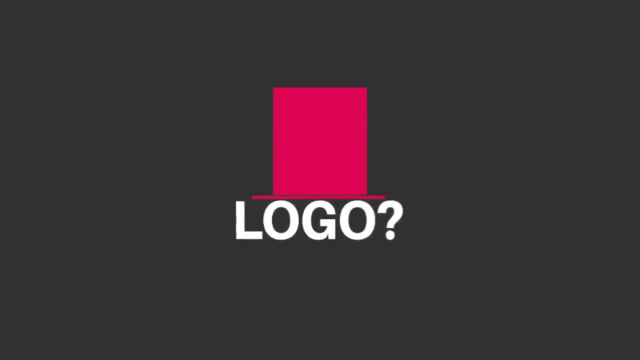 color was one of the two that you chose to use, and tru can follow the right color for your logo. and should you even follow these conventions? well, firstly, you should return to the data and the research that you have on your client's brand, generating keywords linked. 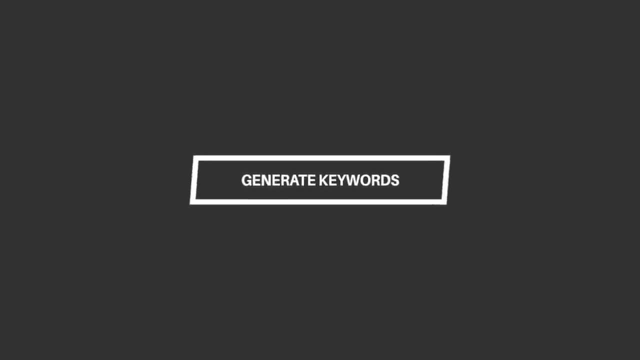 to your brand is essential to the color that you choose. understand the brand and also the typical custom of that brand, and then you can target them with the right colors. let's look at a famous example, and that would be Cadbury, the chocolate company. a recent study showed that 78% of people 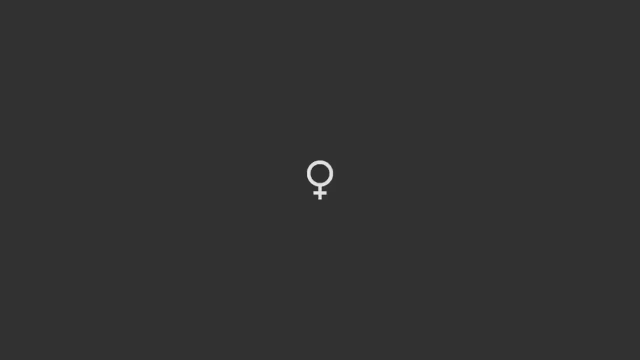 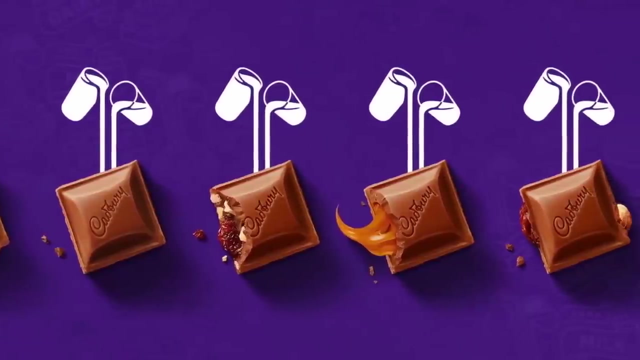 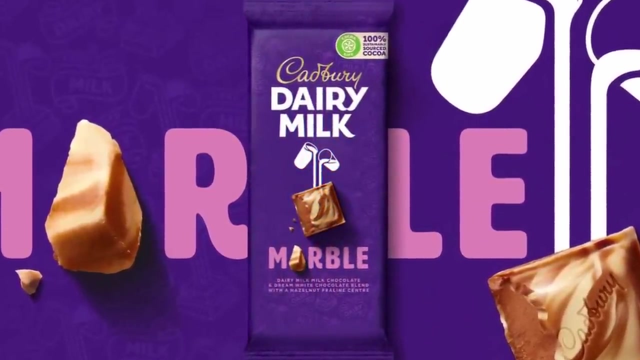 who heard about Cadbury on Facebook were in fact, female. knowing this tiny bit of information is so, so powerful. because what color does Cadbury predominantly use in their branding? if we step back to the color psychology color theory, purple represents luxury, sophistication and even royalty, but crucially, it's a very feminine color. so there's a lot of people out there who don't know. 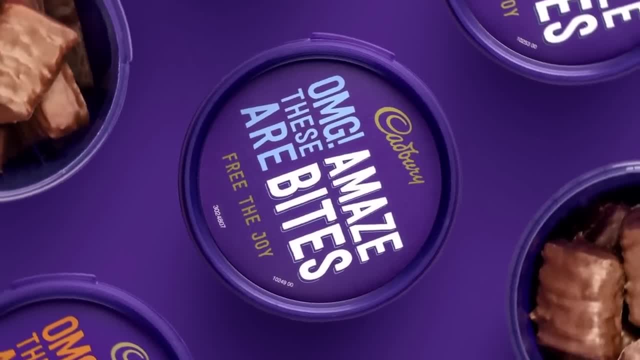 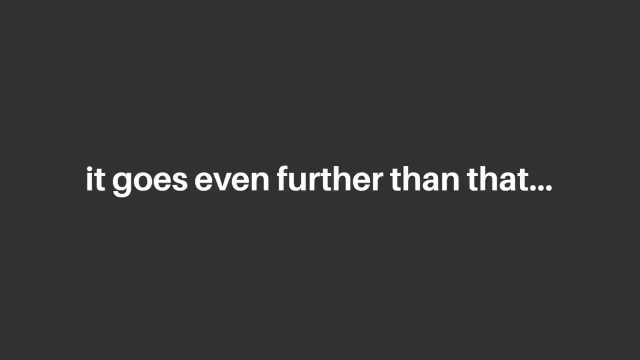 the branding of Cadbury would appeal more to females, which is great, considering what percentage of people who engage with a brand are female. but it goes even further than that in the minds of the consumer, the use of purple elevates the concept of Cadbury as a brand to heights of. 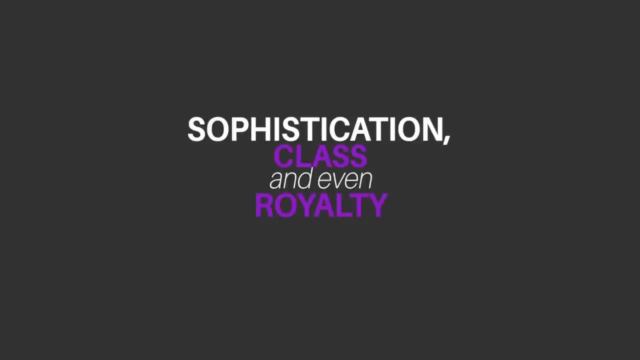 sophistication, class and even royalty. Cadbury didn't just randomly choose purple. it was, of course, a very well thought out and targeted choice, and this is how you should approach a design project: by targeting people with relevant choices. just remember that research is king. but then the question arises: should you stick to just one color? now? me personally, as a logo designer, I rarely use 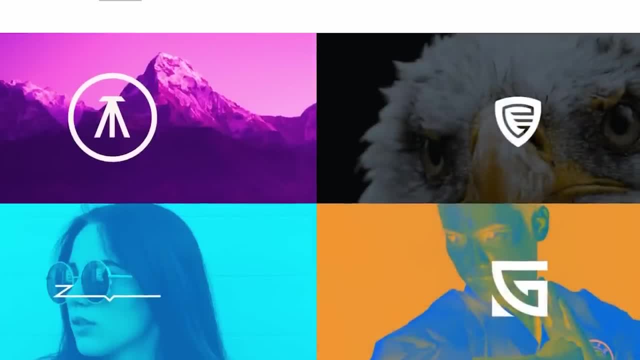 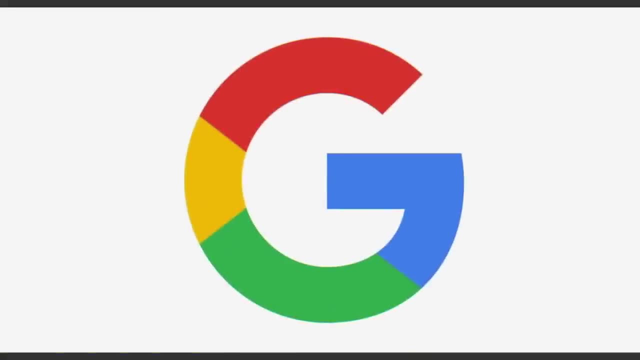 more than one or two colors on a logo. if you are a beginner, then, yes, it is always safe and an easy bet to stick to just one or maybe two colors. but then what about Google or even Microsoft? they have many colors in their logos. yes, these logos for the most. 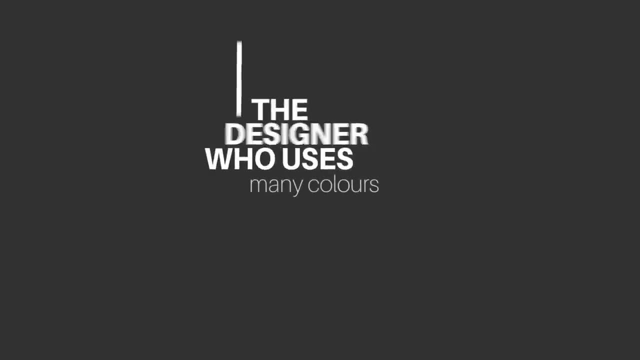 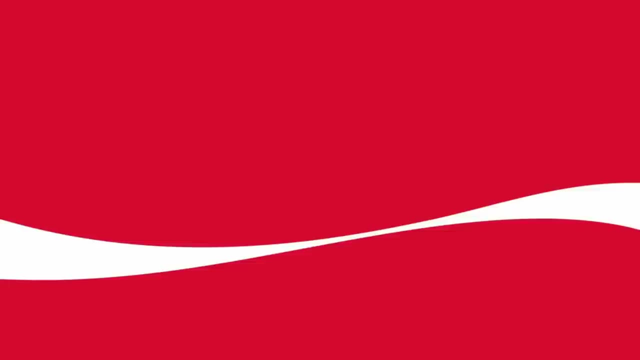 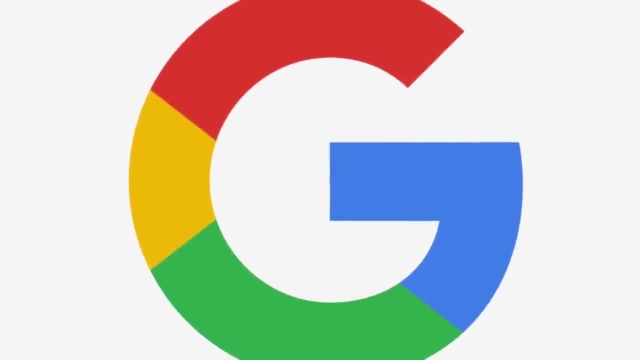 part do work. however, the designer who uses many colors should know exactly what they're doing. going with one color is great for brand recognition and strength. an example here would be Coca-Cola with their red branding, but using multiple colors might be a good idea to stand out from the crowd. the thing is, it needs to be used in a well thought out manner, which often 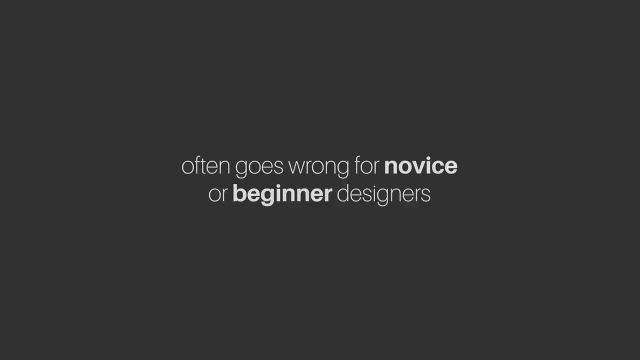 goes wrong for novice or beginner designers. an example here would be the craft rebrand. there is a lot wrong with this logo, but the overuse of color is one of those things. now color can be used to stand up from the crowd in the right way, but again it needs to be thought. 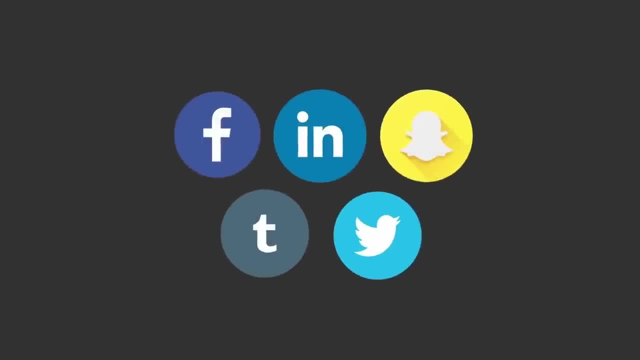 out and planned. if we take a look at social media, you will notice that many logos or apps do use the color of blue. so we have LinkedIn, Twitter, Facebook, Behance, Tumblr and so on. but then we have some outliers, and one of those is Snapchat. Snapchat decided to go. 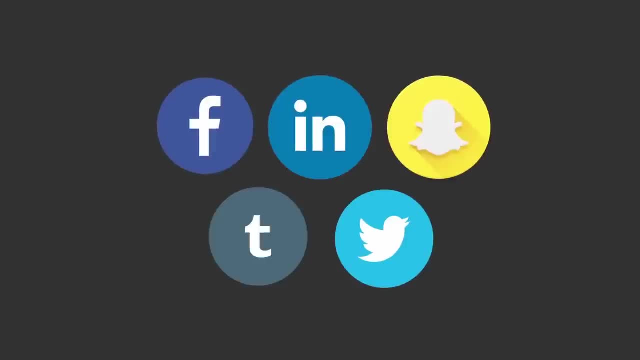 for yellow as the main branding color, which for sure makes them stand out of the crowd. imagine if Snapchat used blue on their logo. it probably would become somewhat lost in the sea of social media branding. so something else you need to keep in mind when choosing colors for your logos is to 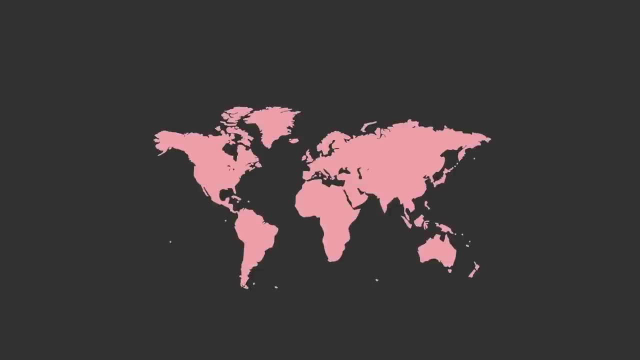 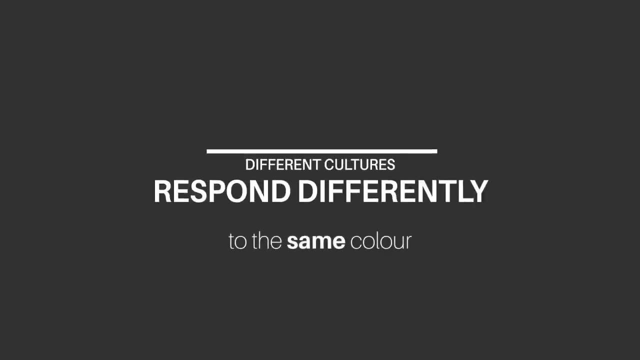 understand where in the world your client is based and also where the Target Market calls home. now why is that important? well, because different cultures will sometimes have different reactions to the same color. this, in the West, can resemble pure and a clean design, whereas in parts of Asia it 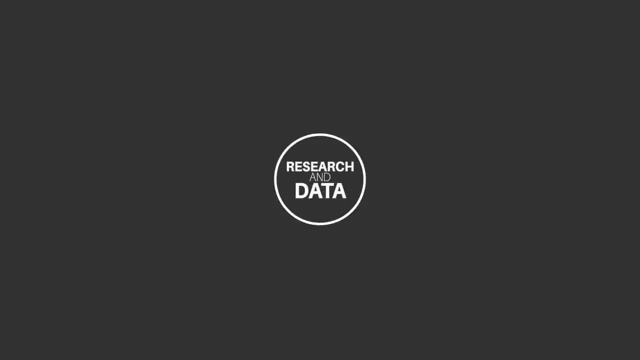 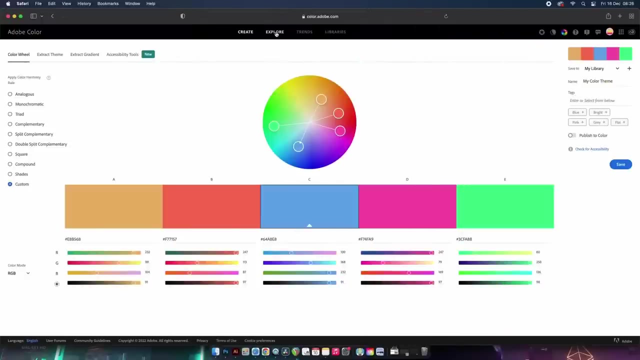 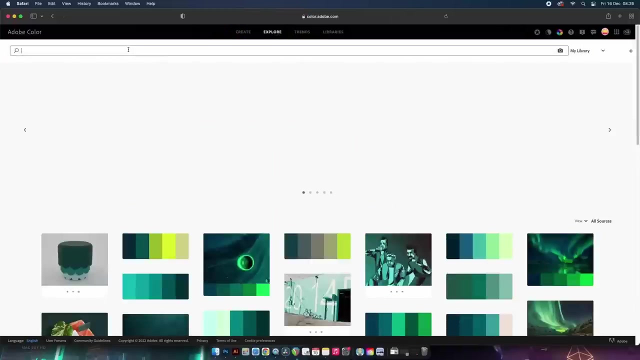 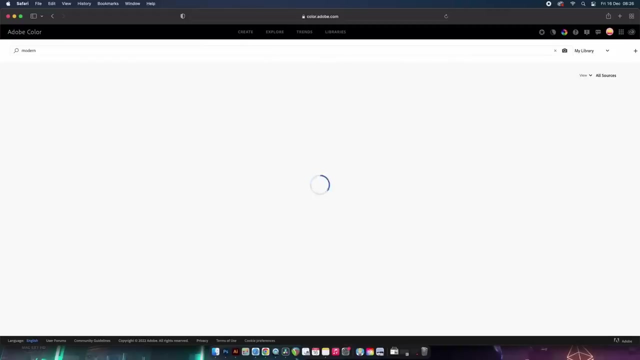 can represent death. so, again, this comes down to research and just data gathering. simply coming to Adobe color, which is totally free, and then head into the explore option, here we can type in relevant keywords from our brief and our client research and this will help us decide on relevant color schemes for our designs, as an example. 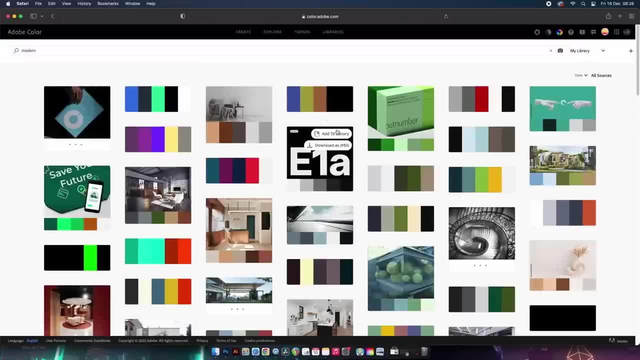 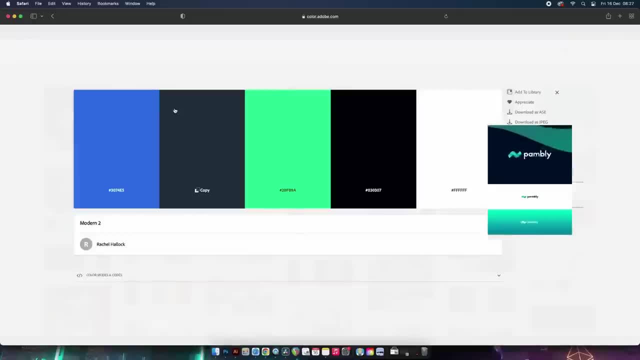 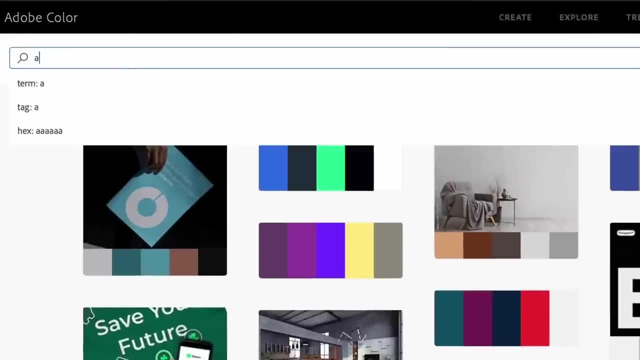 if I'm designing a logo for a kind of modern tech startup, this color palette right here would be possibly a great idea. in fact, I know I've seen such logos use this kind of palette before in the past. when it comes to tech inspired logos, this easy method for choosing colors is so fast. 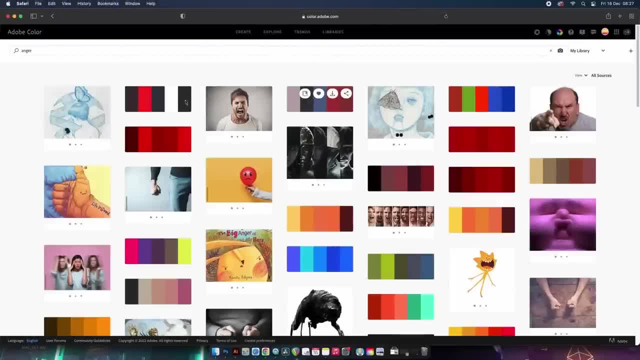 and, yeah, it's pretty easy to do, not to mention really highly targeted towards our audience, if we've done the correct research. the best time to use this tool is probably on logo designs or branding projects, or just when you want to evoke a very certain emotion to the 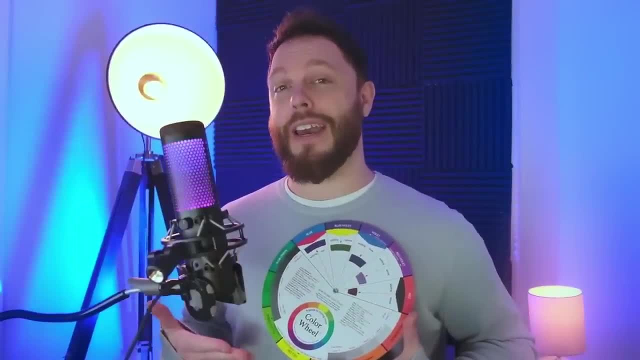 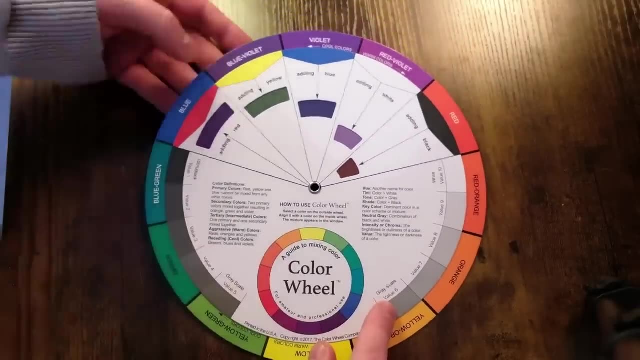 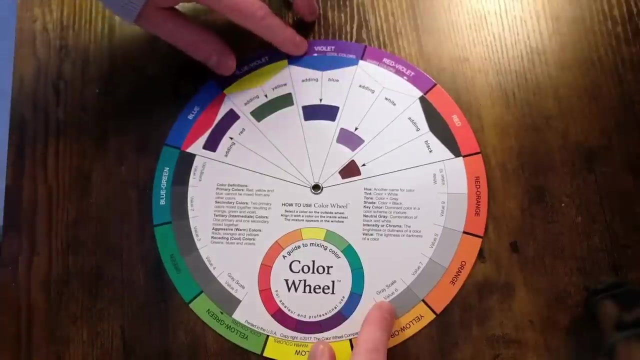 audience. but what about this color wheel here? well, I got this thing a long while back on Amazon and I think it was about ten dollars or thereabouts, so not too expensive. but yeah, this single color wheel actually does four very important things. firstly, it shows us what colors we get if we add the three. 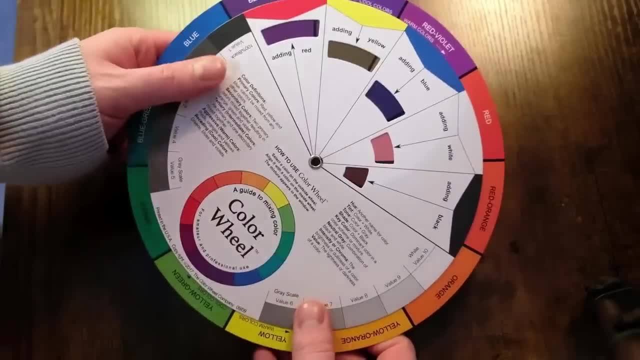 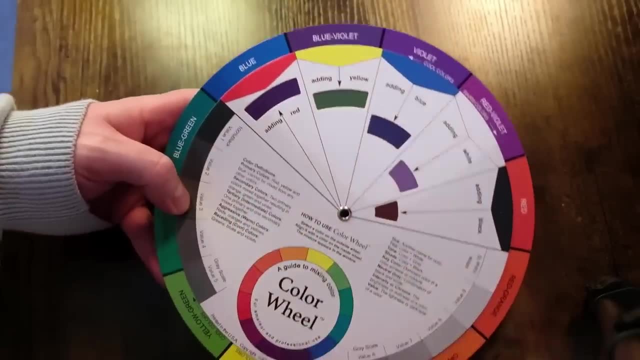 primary colors to another color on the wheel, as well as adding black or white. so here, if we add red to blue, we get purple. as the example on the front here it also shows us from white to black, in grayscale as it's printed out, found along the bottom. and all of this is just 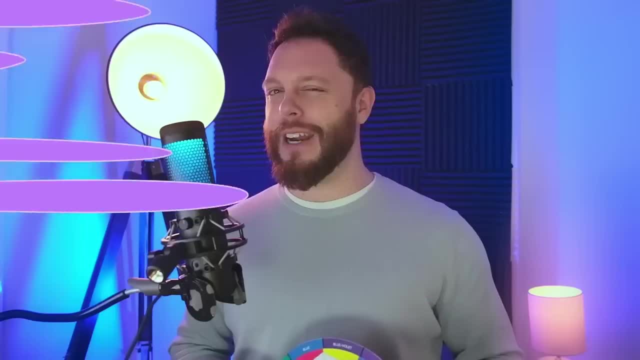 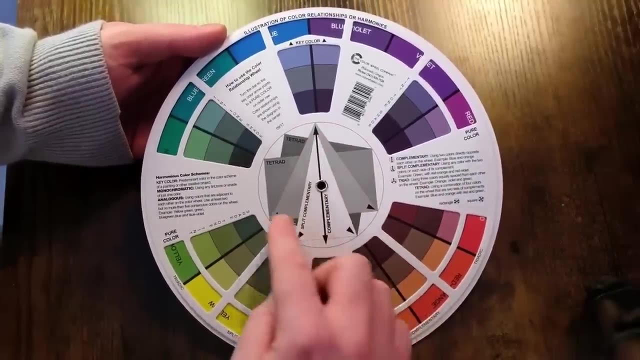 really good to have when you're designing on your computer at your desk. but the really cool thing is when we go ahead and flip it over to the back. but yeah, firstly, on the back we can see in real time the complementary, the split complementary and the tetrad color schemes. it also goes into detail by 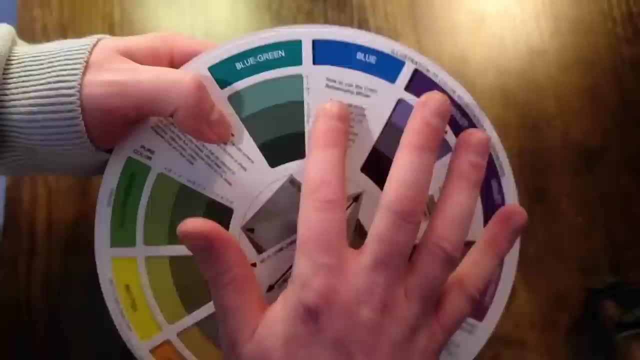 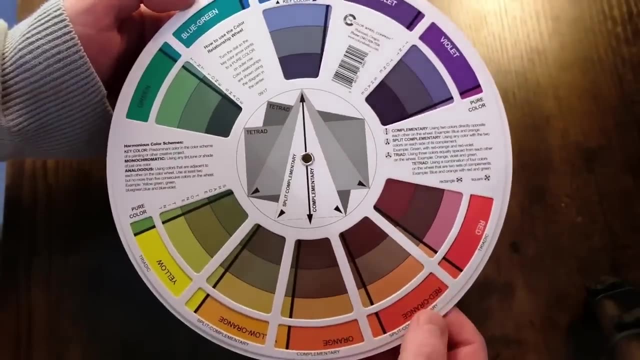 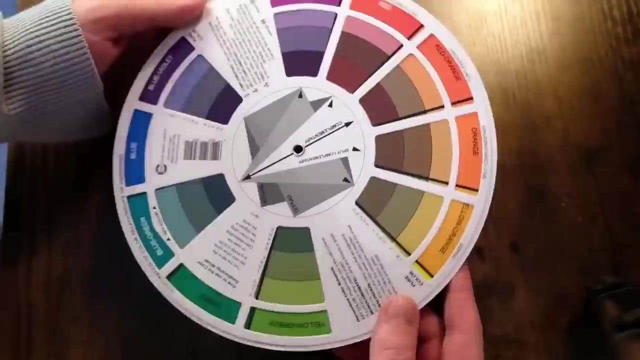 analogous shad and other Harmony good stuff. but if you look right here, we also have tint, tone and shade of every single pure color on the color wheel. this thing is really handy for people who learn in a hands-on kind of way. it's also good to have at your desk when thinking about print design work. 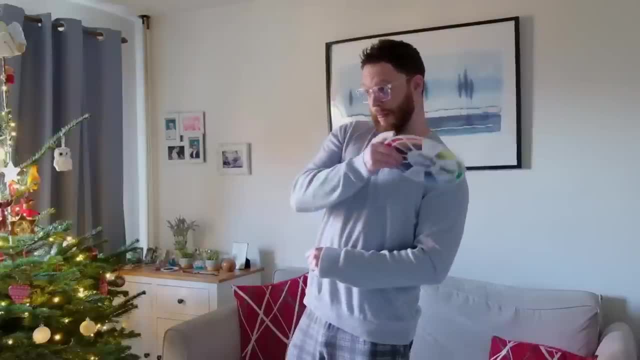 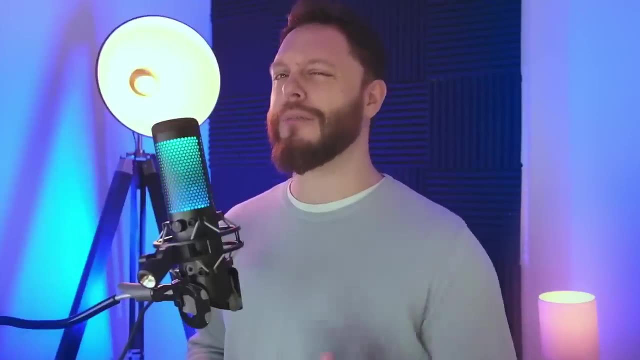 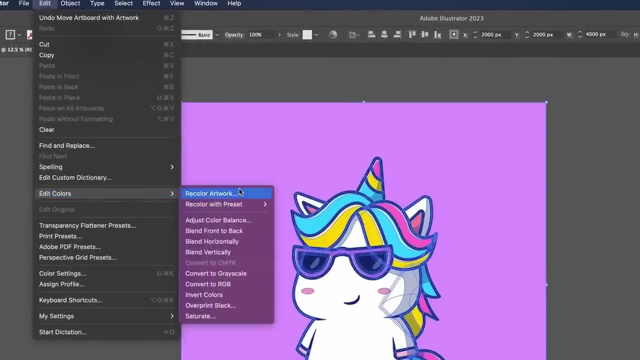 and it also kind of doubles up as a Frisbee, maybe not. the third tool that is used for color and which designers probably should be using is color directly into Adobe Illustrator. when we come into the edit colors menu and go to recolor artwork, make sure the link icon is checked and then we can experiment by shifting the color scheme. for 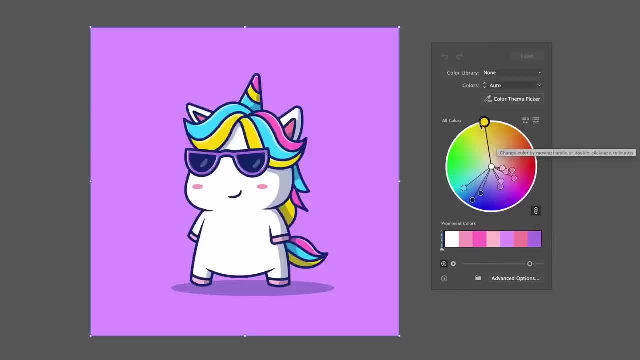 a single design as a whole. you can, of course, unlink the selection to move around single colors, but if you want to make quick variations of a color scheme, of an entire design, this is perfect for that kind of situation. now here's the next tool we're going to be using for something that's going to be done in the next video, which is the color scheme of a color scheme. if you want to make variations of color by using this whole video of color scheme of an entire design, this is perfect for that kind of situation. 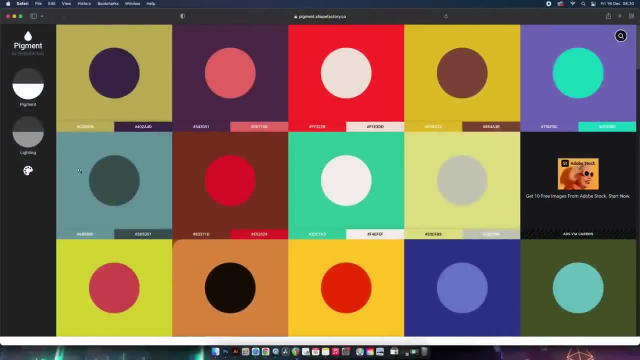 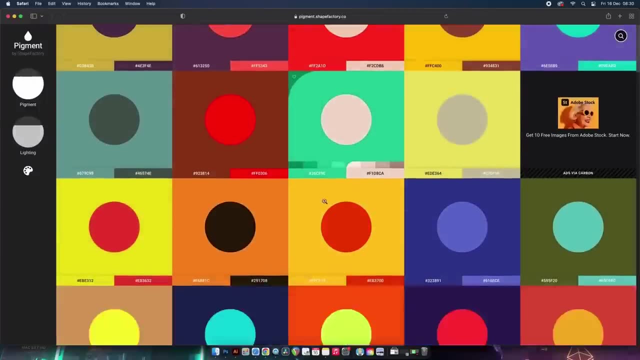 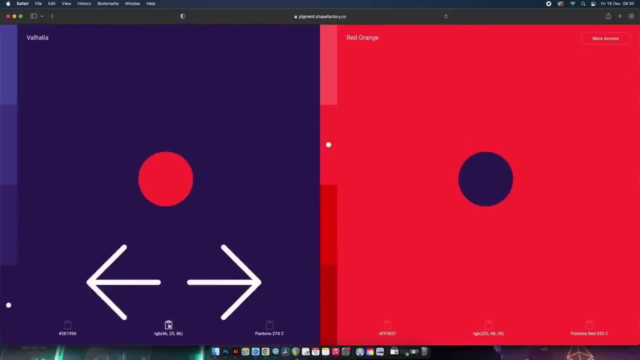 color use and it's called pigment. on the left, we can quickly change the brightness and saturation of the selection and then hop into something we like. the look of this is where this website really comes into use. you'll notice, at the bottom we have the hex code, the rgb values, but also the 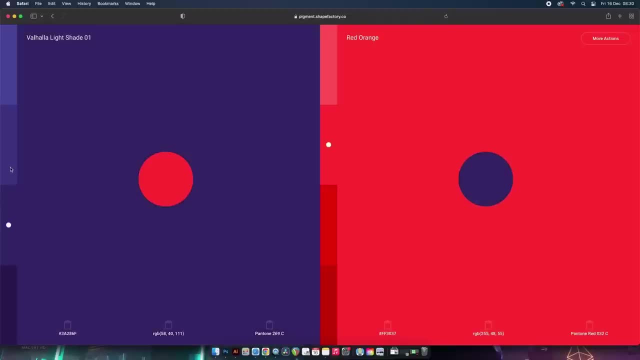 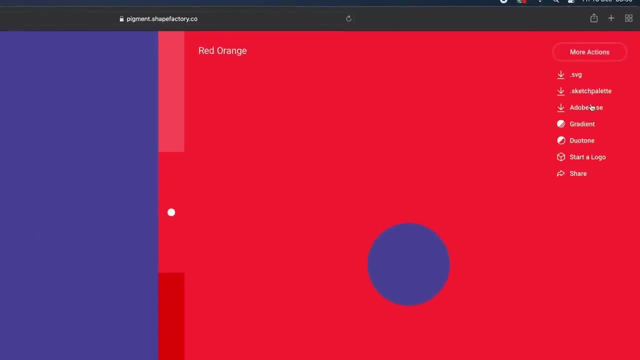 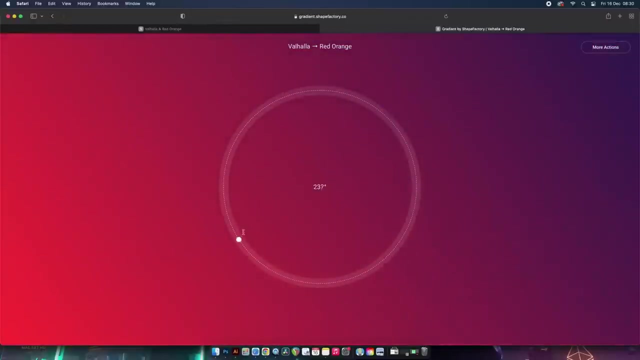 pantone, which is really useful, and if we come up here and click more actions, we can see that we're able to download the color choice to three different useful file formats. we can create and control the direction of a gradient using just the two colors and we can create a duotone image with these two colors, which is pretty cool. 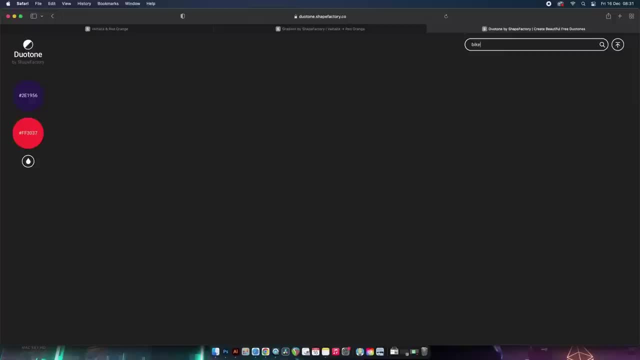 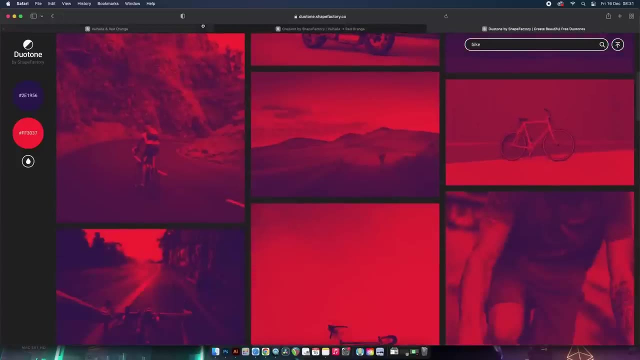 we just need to search in the search bar, find an image and apply the color as a duotone, and of course, we can also share the color scheme to somebody else. now let's not talk about the other option on there, which was use a logo maker with those color schemes, because the less 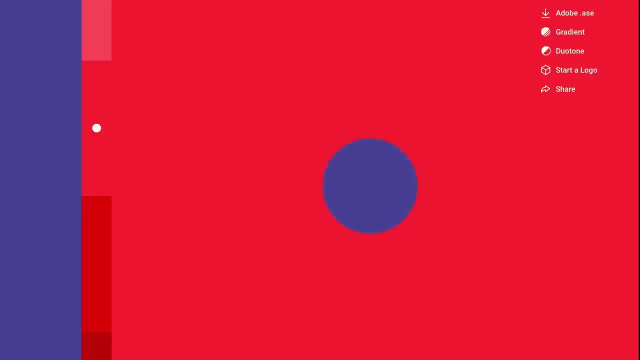 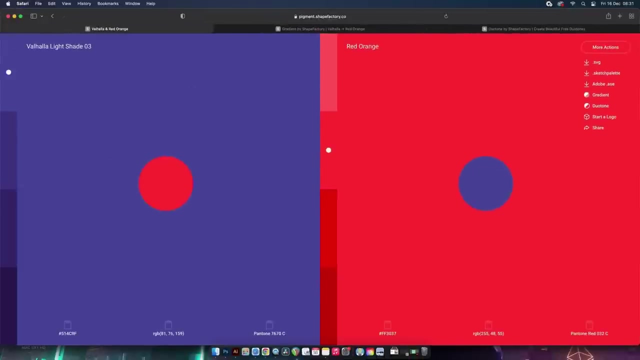 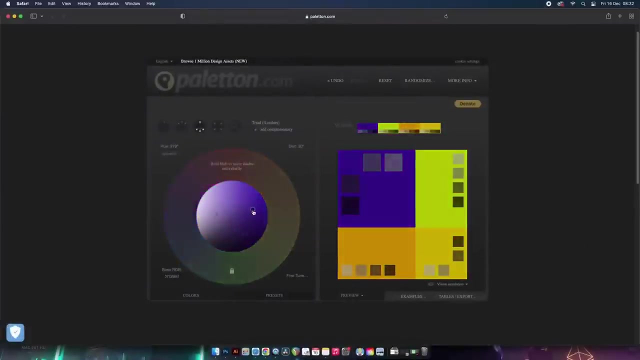 set of logo makers. probably the better. but yeah, this tool is best used for those who want a quick and intuitive way to make a cool duotone color scheme for your next project. and the fifth tool today is a bit more advanced than the previous one. paliton can look a bit confusing when you first 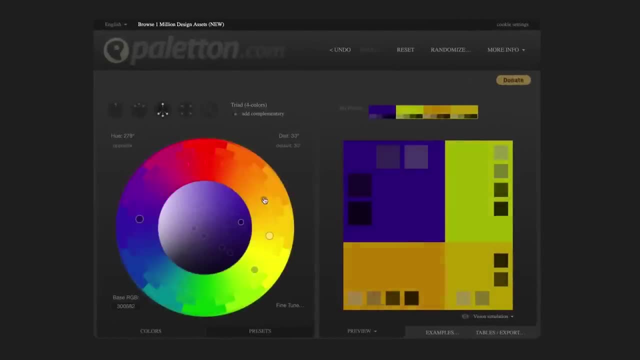 open it, but here's the main use case for this thing. now we can do conventional stuff for creating color on the wheel and then off to the right we have color options related to those harmonies with the hex color codes and so on. however, if we come up to the examples here, we can see our selected color. 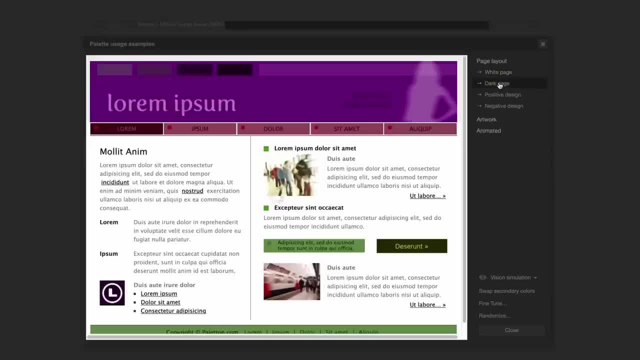 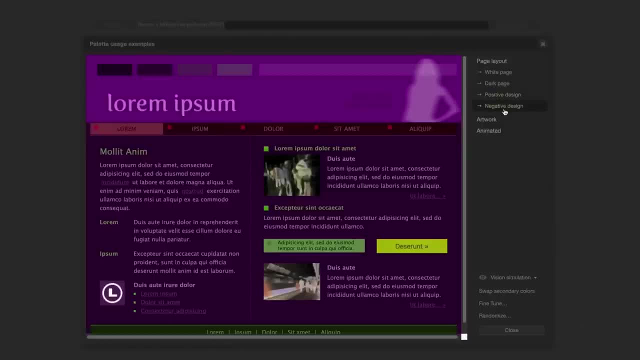 scheme and how it might function on real life projects. firstly, on a website design which- yeah, let's be honest here. this web page looks like it's straight up from the 1990s, but it is cool nonetheless. i'm sure you would agree on that, and then we can see it right here. on some animated: 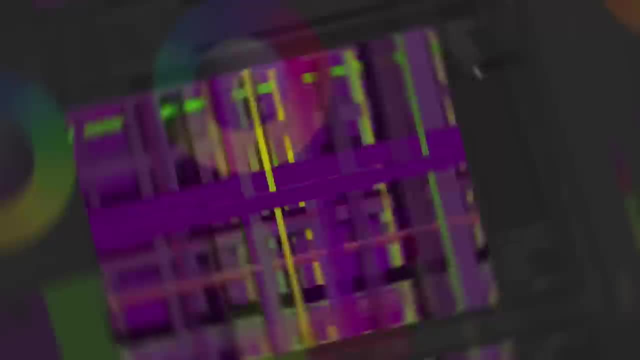 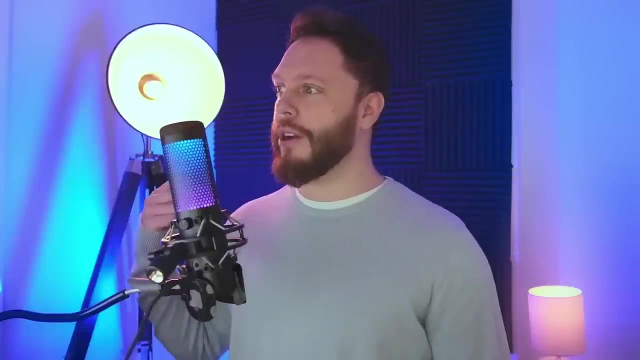 graphics as well. we can see that we can create a color scheme for the color scheme, and then we can also export our creator palettes, which is always handy to have, of course. moving on, we're going to look at a photoshop trick that will save you heaps of time. 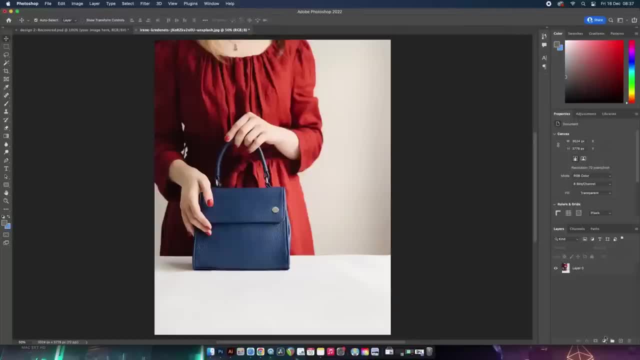 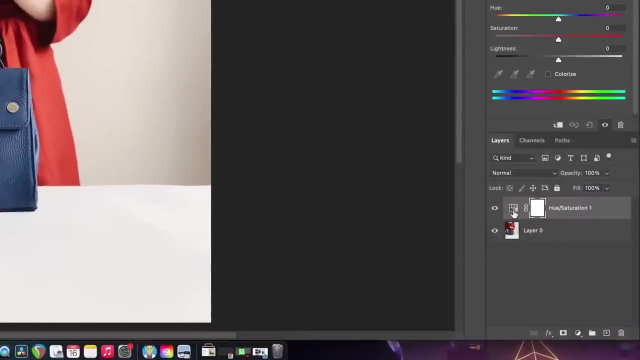 and will really help when using color. now. i first heard of this from the great piximperfect some years ago. if we want to change the color of an obvious selection on our image, we don't need to use any masks at all. just simply go ahead and make a hue saturation adjustment layer and then 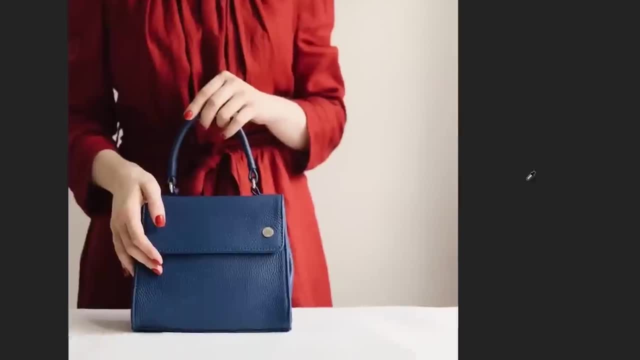 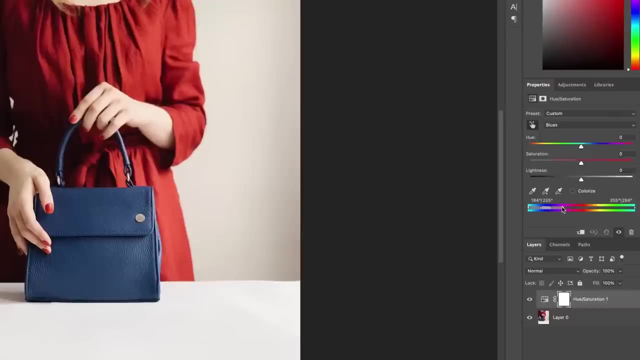 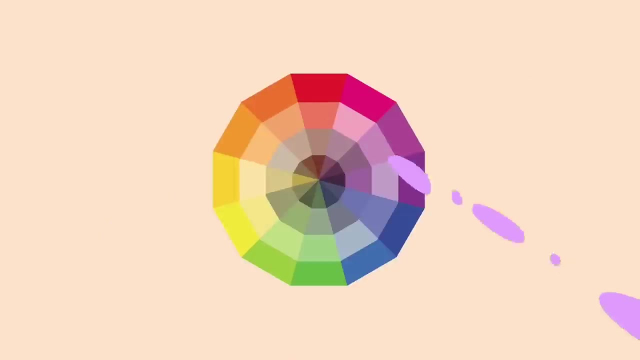 have it. select this tool here and sample your desired color. once selected, you'll notice photoshop has actually picked it out at the bottom here, which then means we can just go ahead and change the hue of the selection really easily indeed, and of course that's without using any masks. this color wheel in particular is useful because it shows hues, tints, tones and also sanctions colors for different machines. you can always find a custom way of selecting your mask, and then so will you be able to filter your mask with some of the explanations in this video at the end of this now. do you like these tutorials, and would you like some video that you enjoy? think about the video, then comment down below in the comments section. will you like our 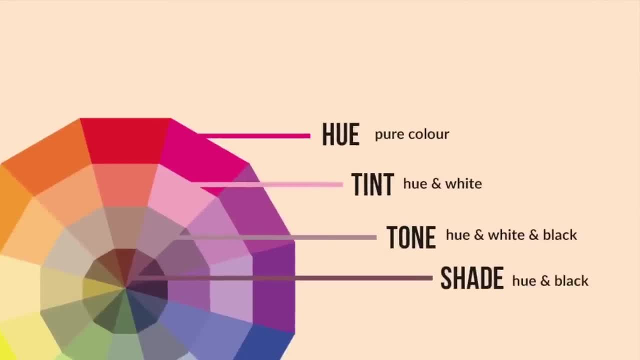 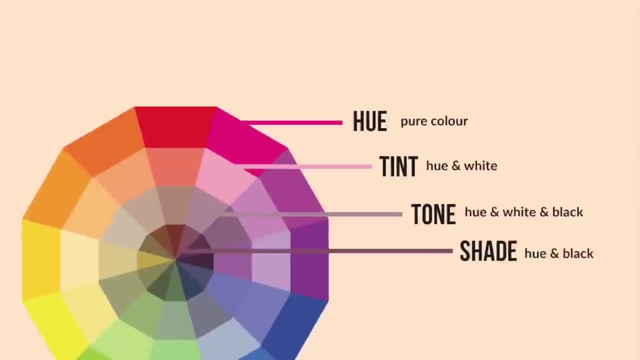 shades. The hue is the pure color around the edge of the wheel, and then the tint is taking the hue and adding a white to it. A tone is the hue plus white and plus black and finally, the shade is the hue plus black. Let's move on to the color. 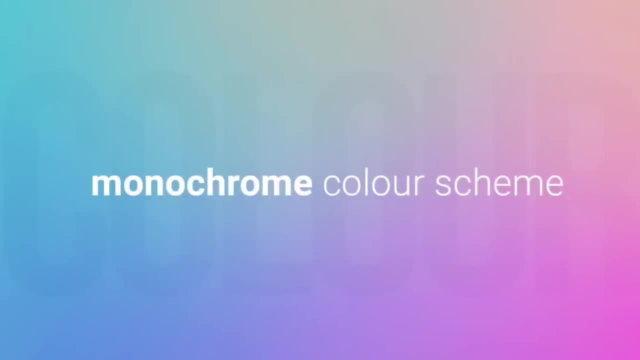 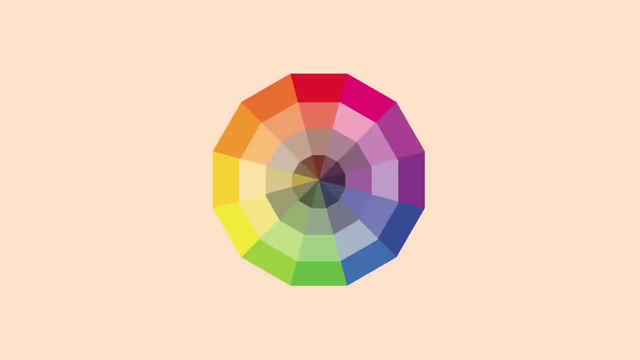 groups. Like I've said before, monochrome is one of my favorite color groups, but it does have a time and a place To make a monochrome color, select a hue and then add some black or some white to the hue, ie a tint or a tone or a shade, and 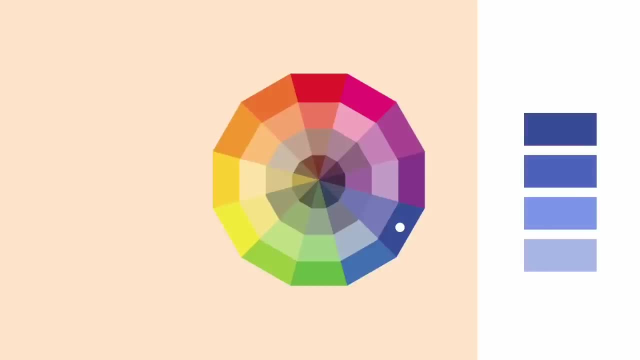 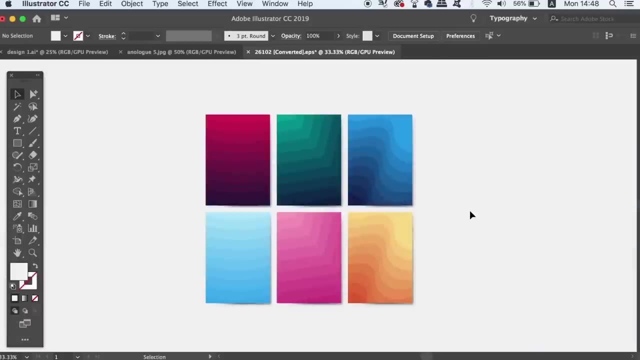 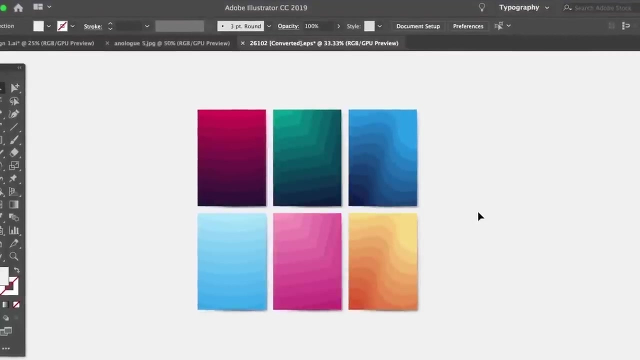 then generate a color spectrum by using that one hue. The thing about monochrome color schemes is that the eye viewing it brushes over them smoothly and softly because there's no real contrast in color. So it's very relaxing and very appealing to the eye. but this means that your design is not going to. 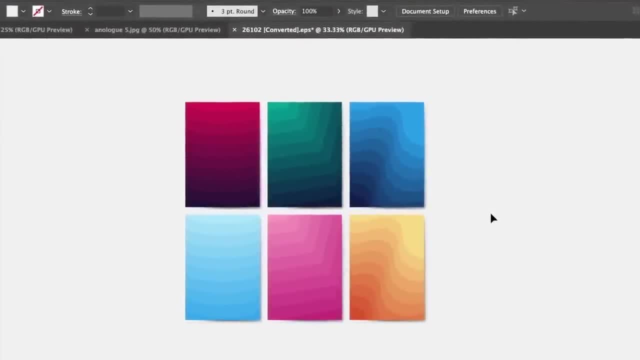 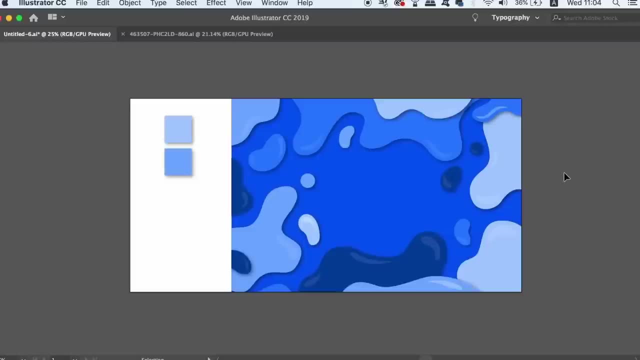 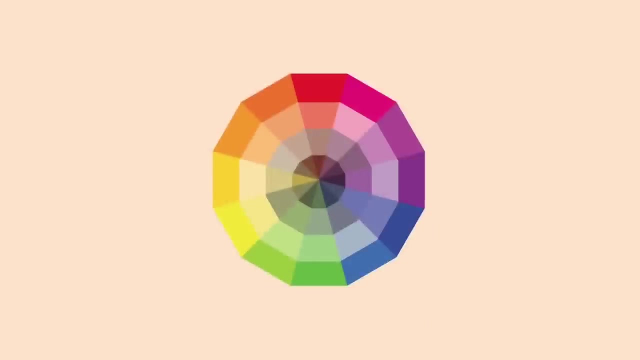 pop, so to speak, and so it's not exactly attention-grabbing. That should suggest that you shouldn't use this color scheme for designs that warrant urgent attention, so like signs or charts and stuff like that, But I find it's very good for digital arts and certain logo designs too. Complementary colors are: 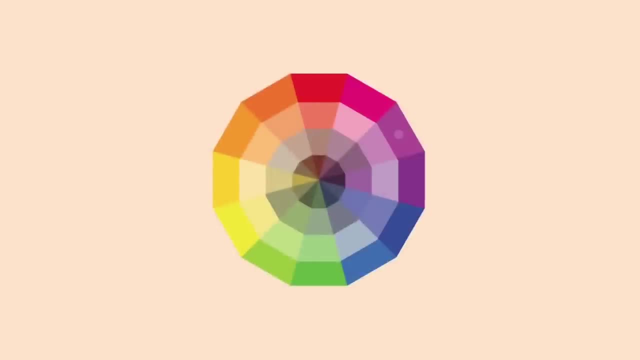 maybe the easiest to understand. You simply select one hue from the color wheel, locate the direct opposite of that colour on the wheel. It doesn't have to be a hue, though. you can use a tint, a tone or a shade, but the key is to locate the direct opposite of that colour. 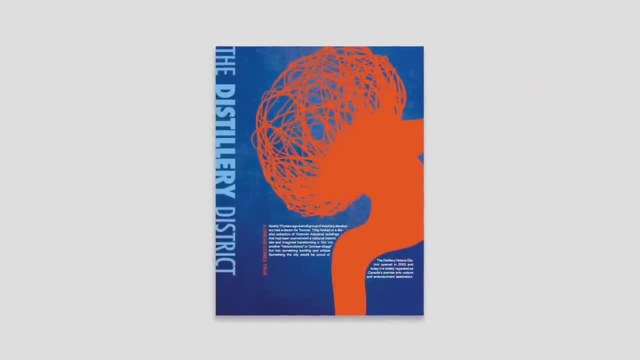 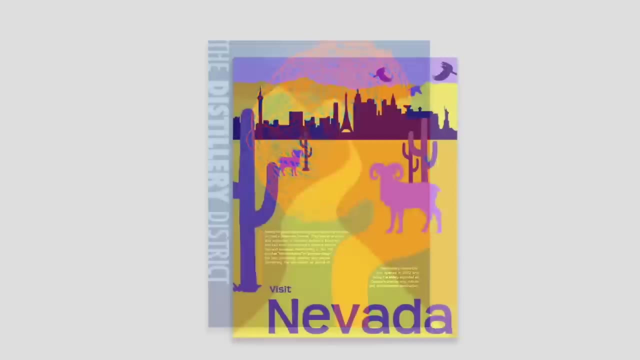 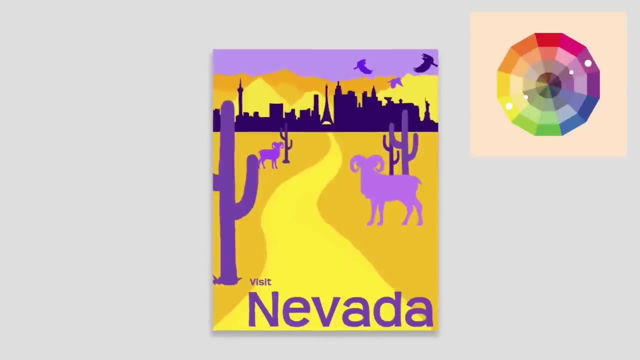 Unlike monochrome colours, complementary are totally contrasting, which means they can be jarring on the eyes, but they do grab attention. Also, there is something appealing to the eye about them. when using designs, however, you need to use them with caution. Try and use like a hue and a tint and then complement that hue and that tint to have. 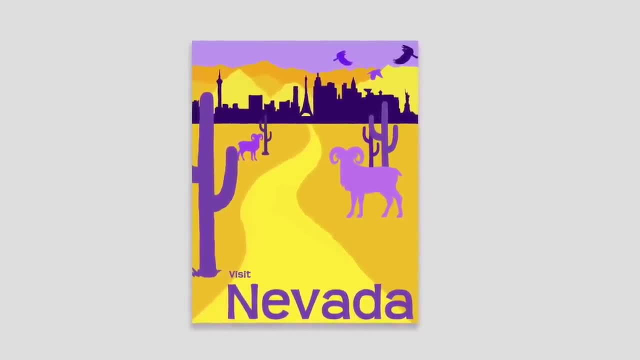 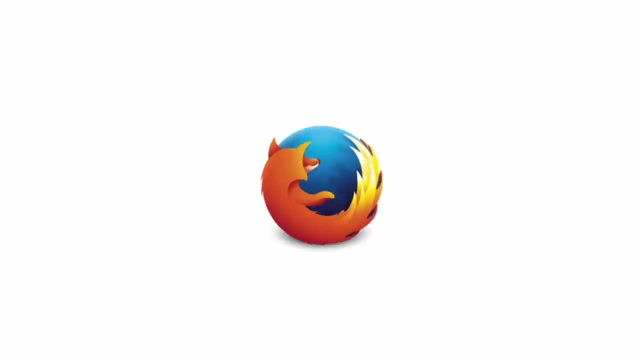 four different colours instead of just two. This gives the design more depth and it's not going to be so jarring on the eyes. A famous design that uses this scheme is the Firefox logo, and also, notoriously, the drink. Fanta uses a complementary colour scheme too. 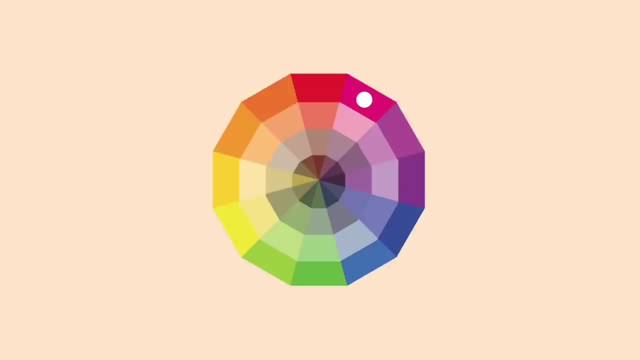 Analogous is where you take one colour on the base colour and then choose a colour either side of it on the colour wheel. This is a three colour analogous scheme, but if you want to use five, just choose two more either side of the first selection. 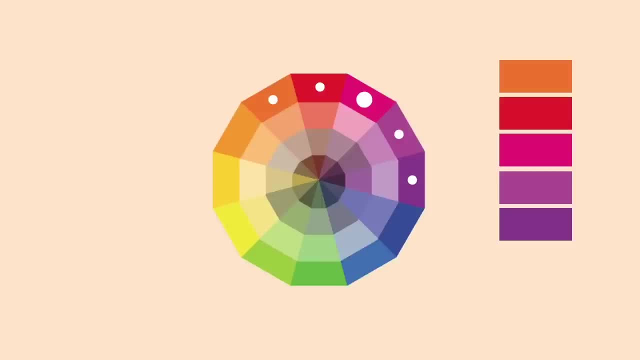 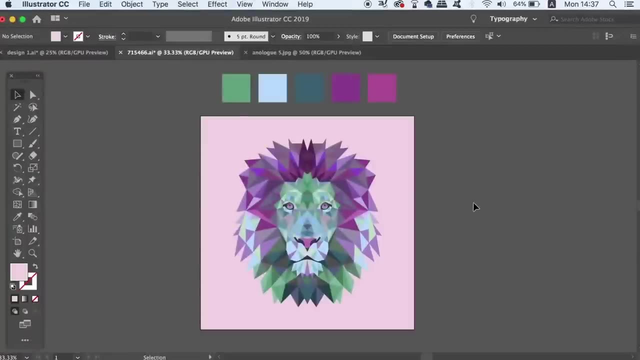 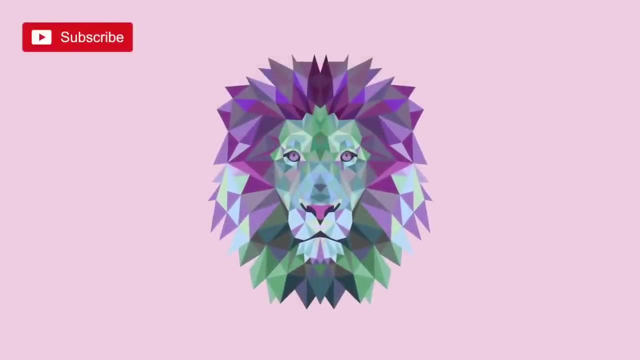 Much like monochrome colours, analogous do not have much contrast within them. They have slightly more, but they're not exactly complementary, are they? With that in mind, these are again good for digital art, softer designs and specific logos. I personally wouldn't be using them for a sign that says for sale or wants to grab some. 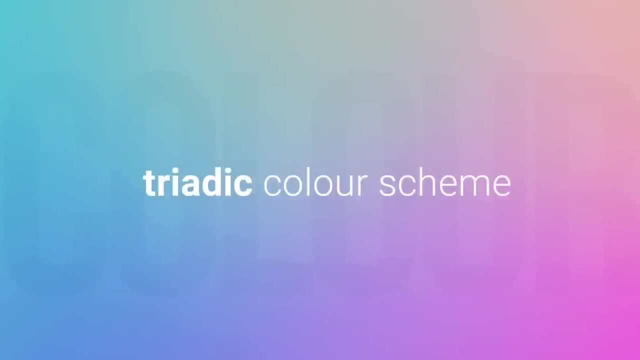 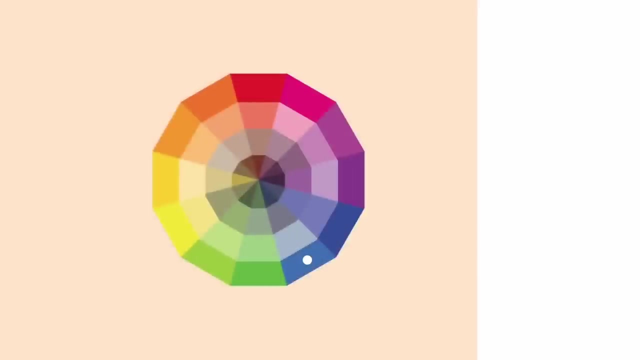 attention. This next colour scheme requires that you find a colour that you wish to use for your design, then move four spaces, leaving three gaps in between, and then do that again around the colour wheel. You then have three different colours evenly spaced out around the wheel.